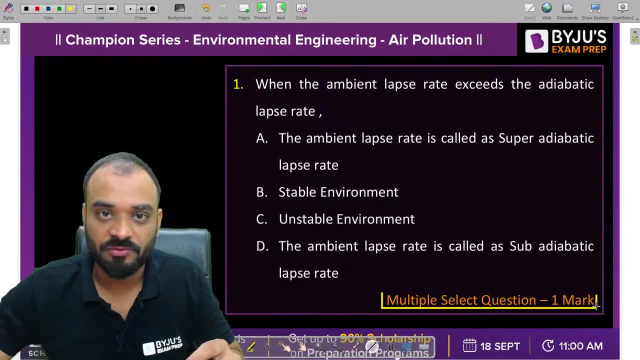 One mark question. Okay, kindly read the question very carefully, guys, before giving your answer. Okay, what is written in the question? Let's understand. when the ambient lapse rate exceed the adiabatic lapse rate, then which of the following option is correct? 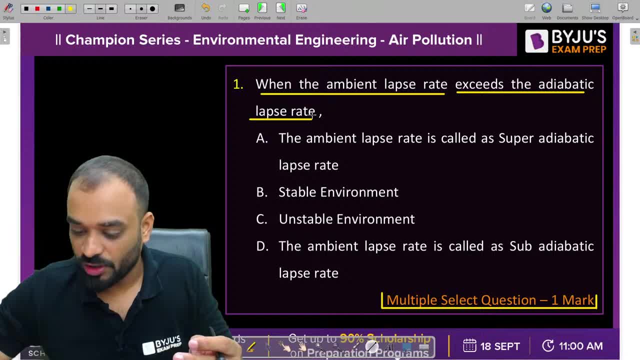 Pretty Anc. Pat Moti, very nice. What about the student? But the ambient lapse rate is exceeding adiabatic lapse rate. Tell me, guys. Motion See that. Mary AC: very nice. What about other students? What do you say, guys? 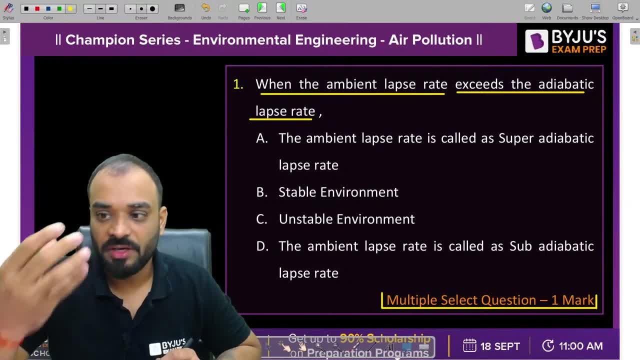 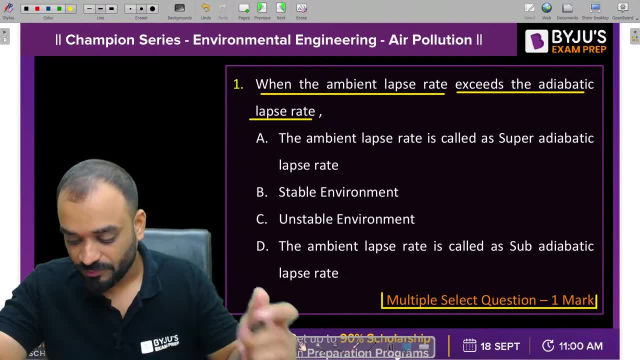 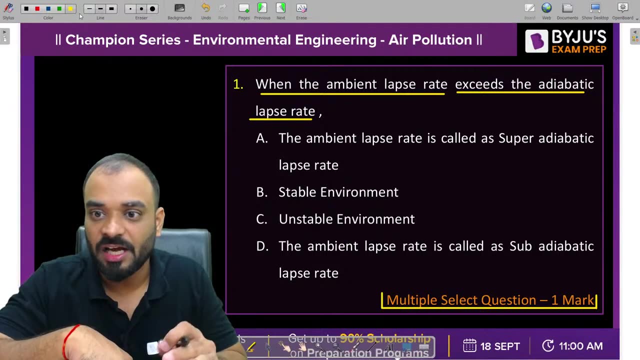 detractors. If environmental lapse rate right, If environmental lapse rate is trying to accessories Goodbye, Take Left here rate, then which of the following option can be correct over here: valley anc. very nice guys, so let's understand this particular problem. let me explain first what is basically your alr and what 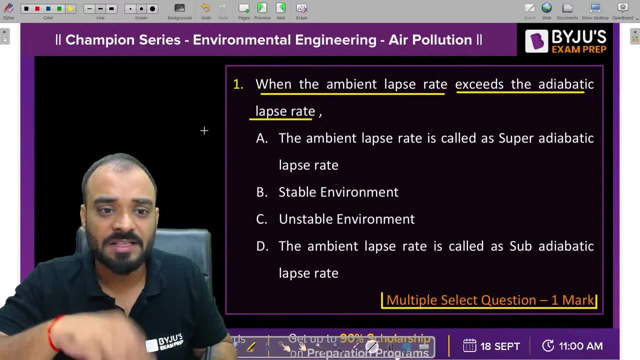 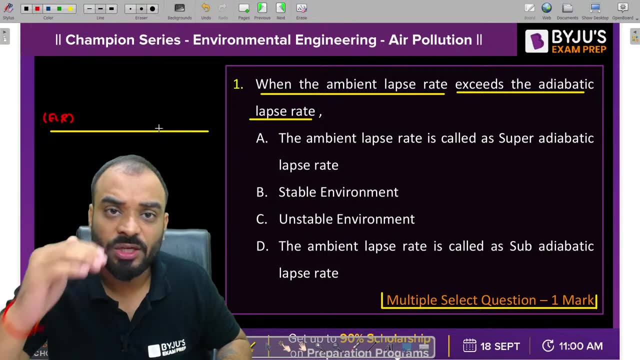 is our elr value? okay, you know that, guys. elr is nothing, as that is basically environmental lapse rate. elr is nothing, as that is basically environmental lapse rate. environmental lapse rate. now, what is environmental lapse rate? you know that, guys. the rate of change of temperature. 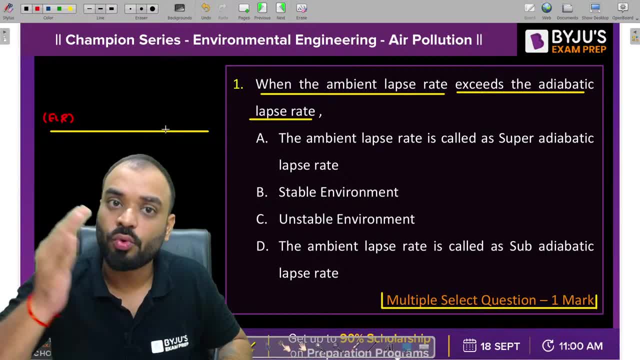 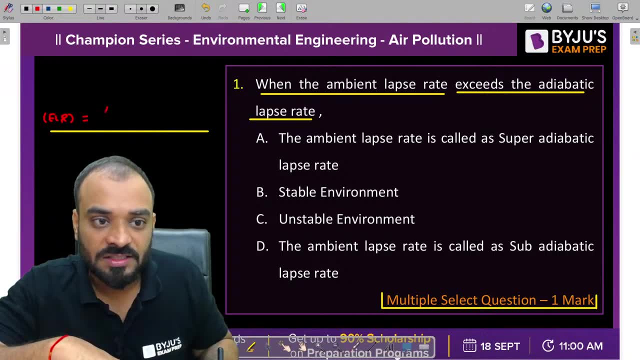 with respect to height by which the environment is trying to cool down its itself. right, that is basically environmental lapse rate, so we can write here: it is nothing as the rate of change of temperature of the surrounding air with respect to change in height. that is known as what that is. 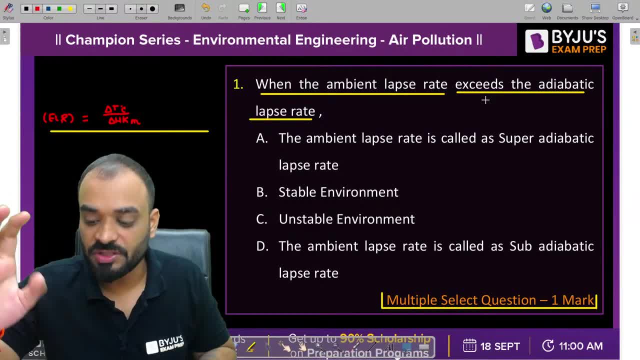 known as elr. now, similarly, guys, we have another term, which is known as adiabatic lapse rate. what is adiabatic lapse rate? you can define it as the rate of change of temperature of an air parcel of the environment, which is the rate of change of temperature of the environment. 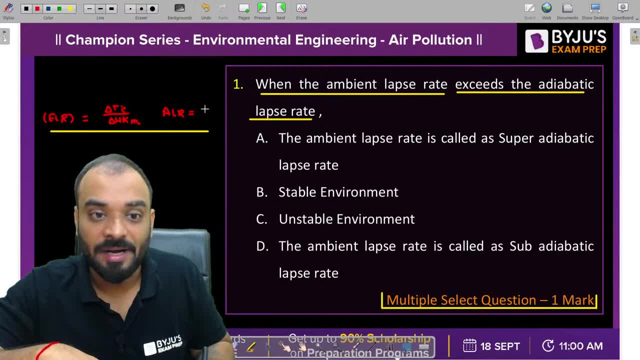 with respect to change in height. that is called adiabatic lapse rate. okay, that is called adiabatic lapse rate. so basically, there are two things: one is surrounding air and second one is what? second one is our air parcel. okay, let us suppose this is air parcel. what is air parcel? this is the air in. 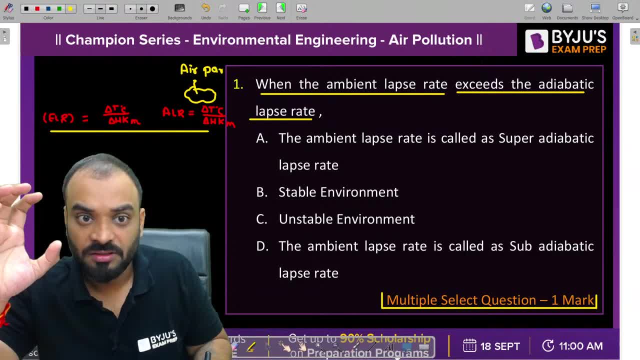 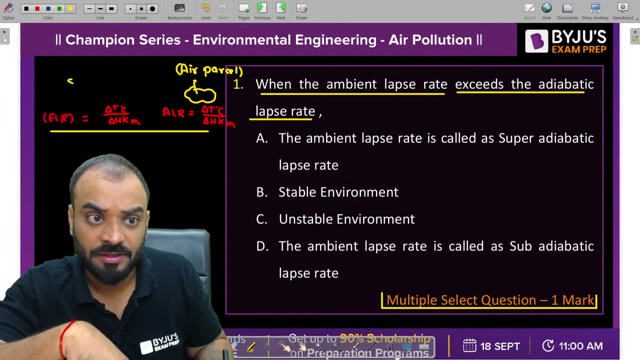 which certain amount of pollutant are present. right, the concentration of pollutant are present in this particular air parcel and surrounding air is nothing as our ambient air, right, surrounding air, or you can call it as ambient air also. okay, sir, now listen guys, what this particular rate exactly telling us this is nothing, as this is the 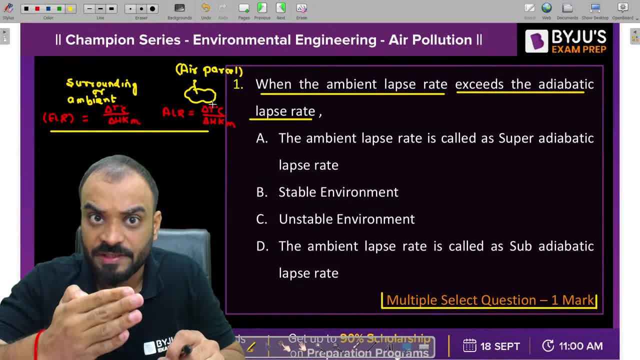 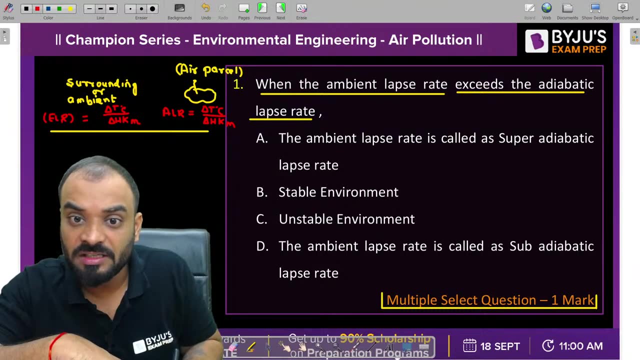 rate by which the air parcel is trying to cool down itself. similarly, guys, we can say that elr is nothing as the rate of change of temperature with respect to height by which surrounding air is trying to cool down itself. now tell me, guys, if this particular rate, which is basically our elr environmental lapse rate, or you 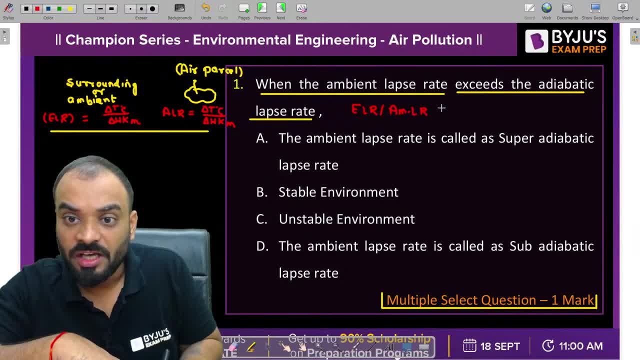 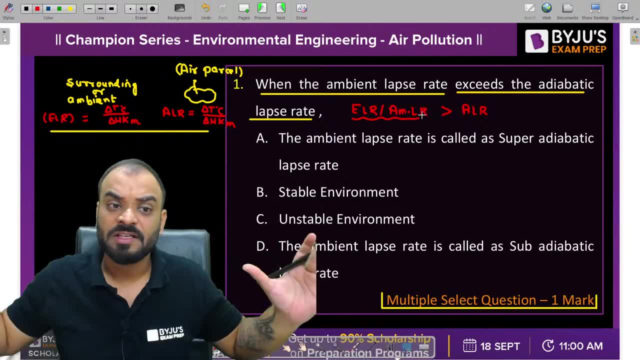 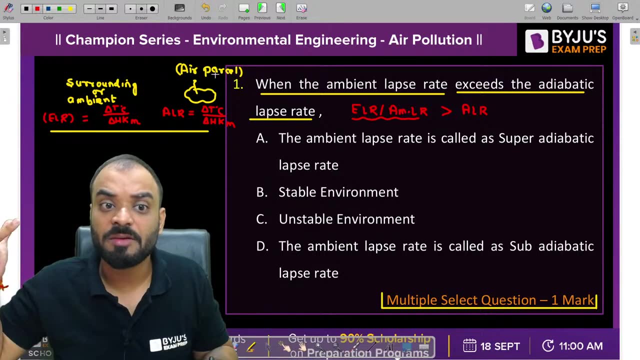 can call it as ambient lapse rate also. okay, if this particular value is trying to exceed the adiabatic lapse rate. so can i say that my surrounding air is trying to cool down early. right, my surrounding air is basically cool one and our air parcel is a hotter one because the rate of cooling of this 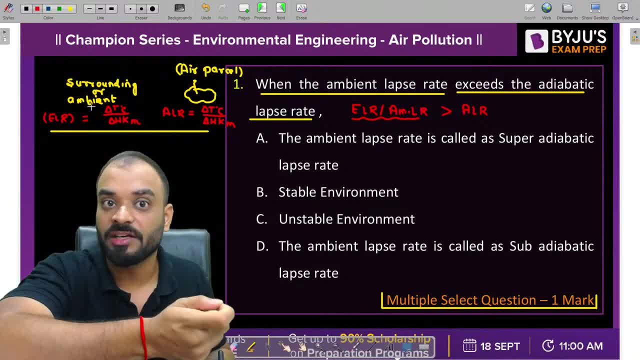 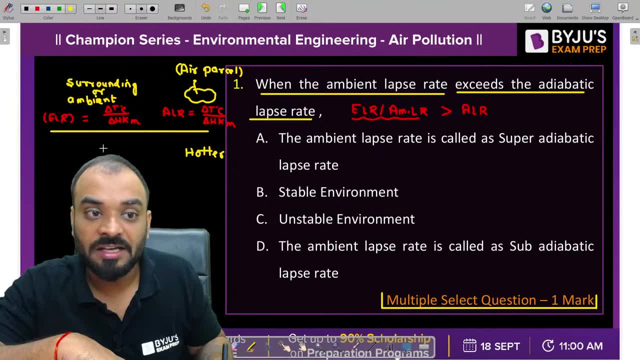 particular air parcel is less than that. so this particular rate is trying to cool down itself. that's why, guys, according to this particular here, the air parcel is hotter if it is at room temperature situation, guys, compared to surrounding air. so we can call it as thegender- the particular rate is: 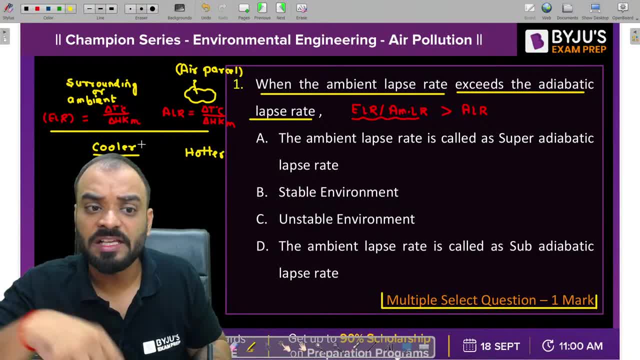 getafe at room temperature. if it is at room temperature which is evenよt the air lower, so if it has preserve particular going to, but рассured by certain level of temperature, is still stayed. and that's whay guys. as compared to same. if the level is less than, as compared to. 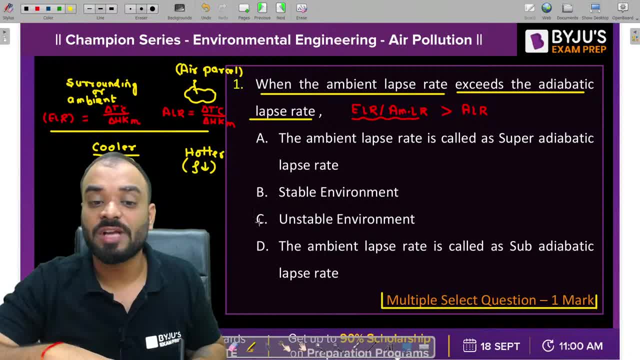 surrounding air and 22уется, a lot less is coming up. so now, hello pues. condition is known as unstable environment. clear, such type of condition is known as unstable environment. now, guys, whenever the ELR value is trying to exceed the ALR, then such type of ambient. 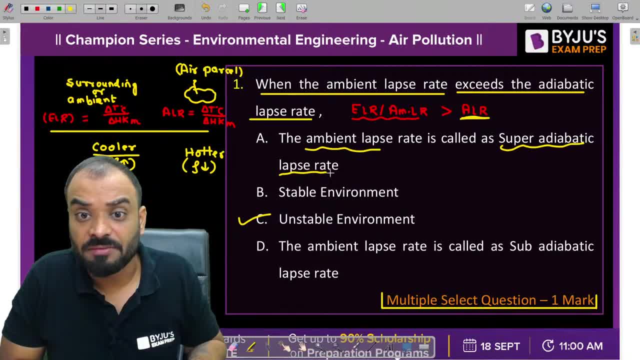 lapse rate is known as super adiabatic lapse rate. please remember this term. if ELR value is trying to exceed the ALR value, then it is nothing as super adiabatic lapse rate, clear. so that's why A and C is the correct answer. and in such situation you may get the unstable environment. 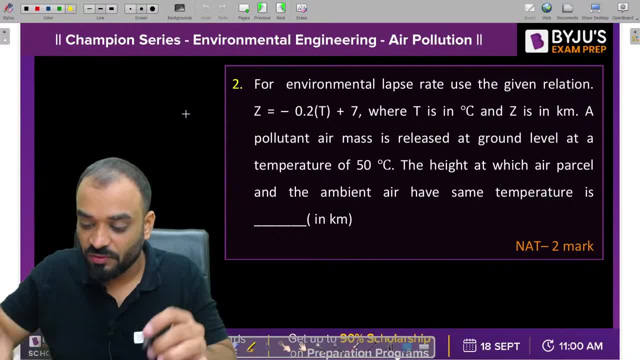 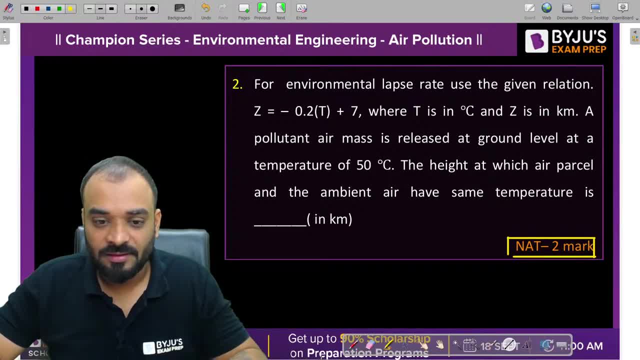 now you just need to solve this particular problem, guys. right, and it is a numerical answer type question. quickly solve it, guys, and let's see how it works and let me know the answer. quickly solve it and let me know the answer. quickly solve it and let me know the answer, guys, what will be the answer for the given? 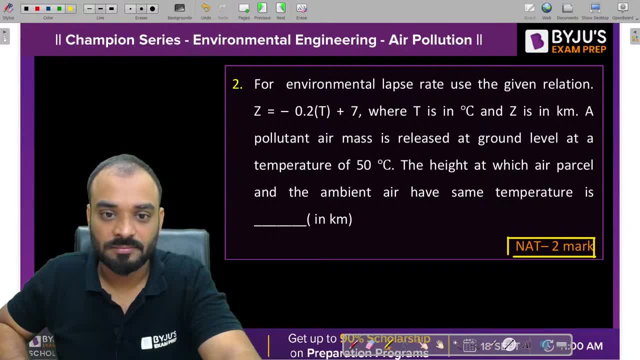 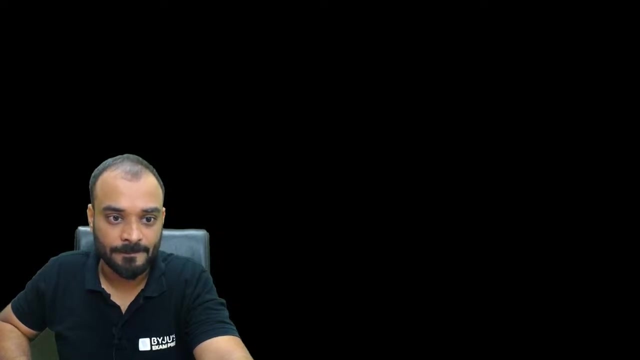 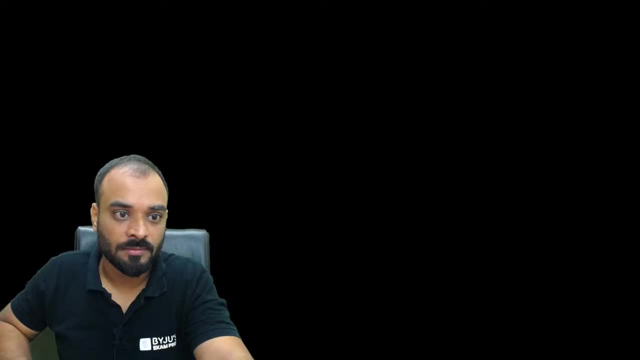 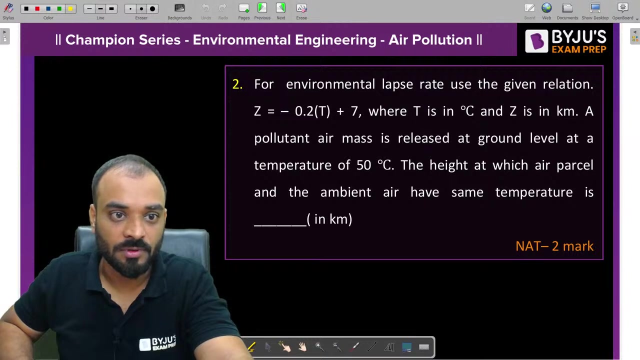 Just hold, guys, just hold, okay, Just hold for a second. Okay, guys, I think now you are able to see this, right Now you are able to see the problem. okay, Now tell me, guys, how we can solve this particular problem which is in front of you, okay. 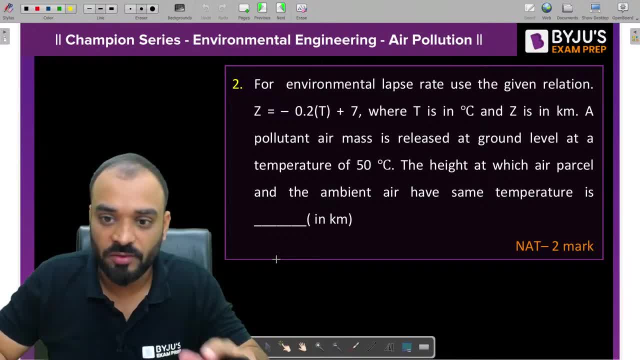 So this problem is based upon what This problem is based upon again: our environmental lapse rate and adiabatic lapse rate. Now this is a numerical answer type question guys, in which we have to solve the problem and we need to find one value over here which we have to put in the question. okay, 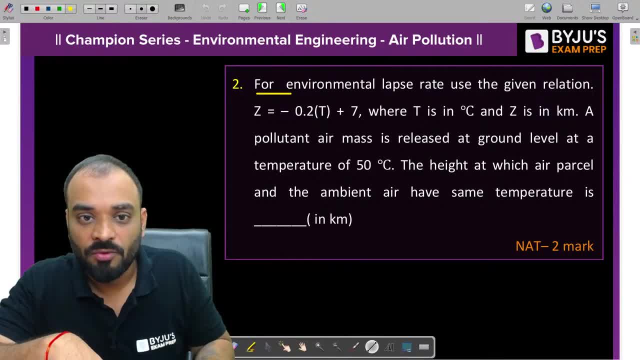 Let's understand the question first, what is given in the problem for the environmental lapse rate. So, for example, if we have a given relation, Z is equal to this one right For ELR value. this is the relation which we have to use and T should be in degree centigrade. 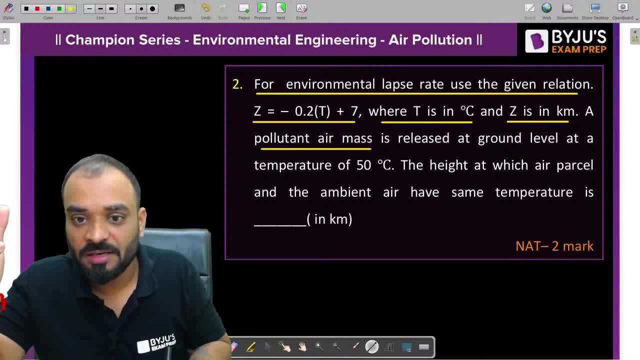 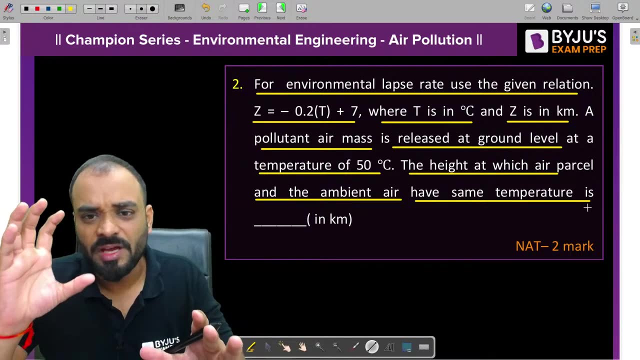 and Z should be in kilometer. Now a pollutant air mass is released at the ground level at a temperature of 50 degree centigrade. the height at which air parcel and the ambient air have the same temperature is Now. what do you need to find over here, guys? basically we are having an air parcel which 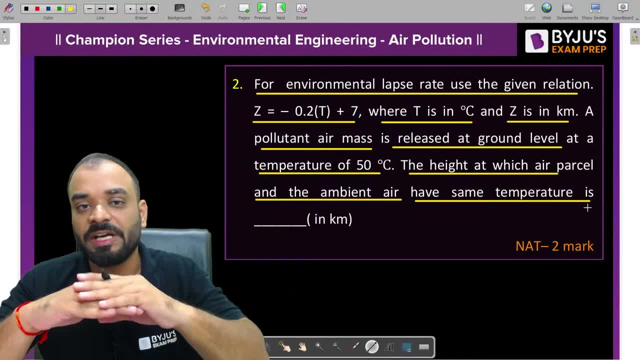 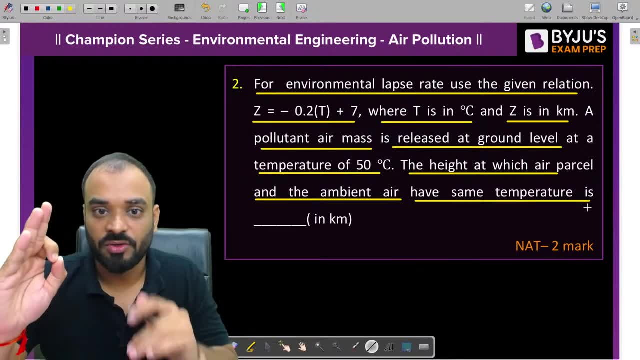 is present at a ground level. Okay, The temperature is equal to 50 degree centigrade. and they have mentioned one equation over here, guys, which is basically for your environmental lapse rate value, That means Z is equal to minus 0.2, T plus seven. 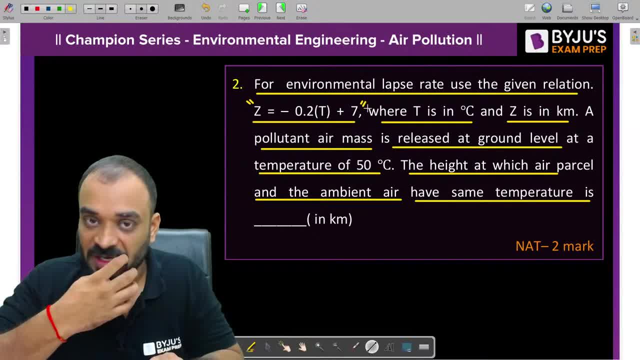 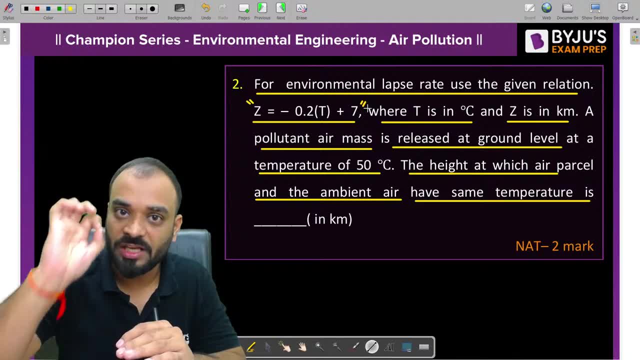 This is basically our environmental lapse rate equation right Now. what do we need to find over here, guys? We need to find the position or the height at which the temperature of surrounding air and the temperature of our air parcel will become same. And that is the question, guys, for this. 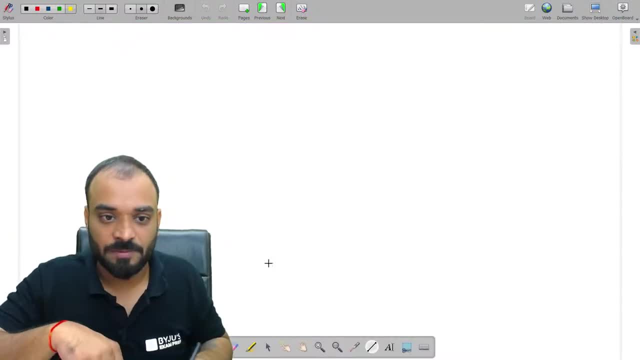 Right. So let's understand, guys, how we can solve it. Let me explain. So let us consider, guys: this is our ground level, This is basically our ground level, and at the ground level we are having an air parcel whose temperature is equal to how much? 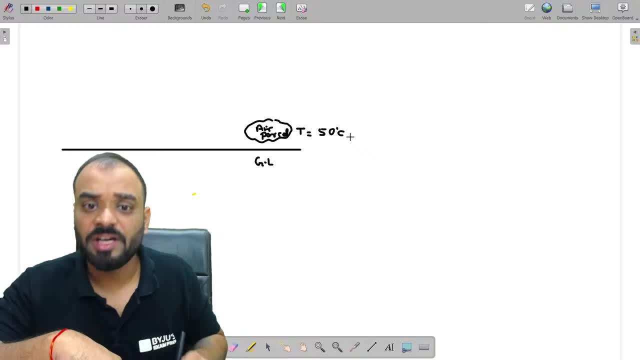 Whose temperature is equal to 50 degree centigrade. Now tell me, guys, do you know the rate by which the air parcel is trying to cool down itself, which is known as dry adiabatic lapse rate? Do you remember this particular value, guys? 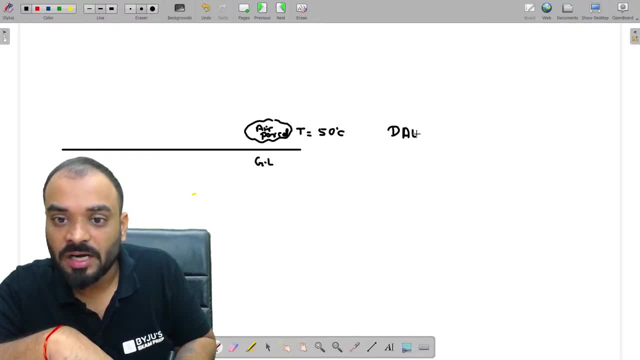 Dry adiabatic lapse rate. dry adiabatic lapse rate. This value is equal to how much? it is equal to 9.8 degree centigrade per kilometer. Do you know that Right? So we need to use this particular rate. 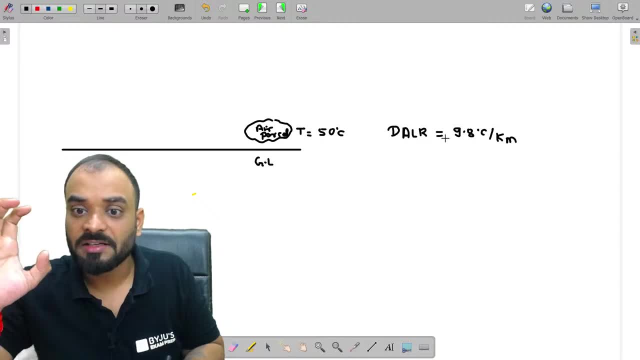 So right now the temperature is 50 degree centigrade, Okay, And the rate by which this air parcel will cool down is equal to how much. it is 9.8 degree centigrade per kilometer. Now let us suppose if this particular air parcel is trying to move upward with a distance. 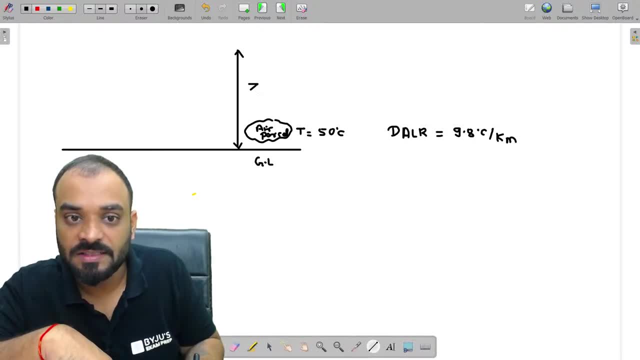 of Z kilometer. Okay, Let us consider this distance is Z kilometer. This distance is equal to how much? Let us consider it as equal to Z kilometer And let us consider certain temperature will occur at this particular point. Now our task is to find out the temperature at this particular level. 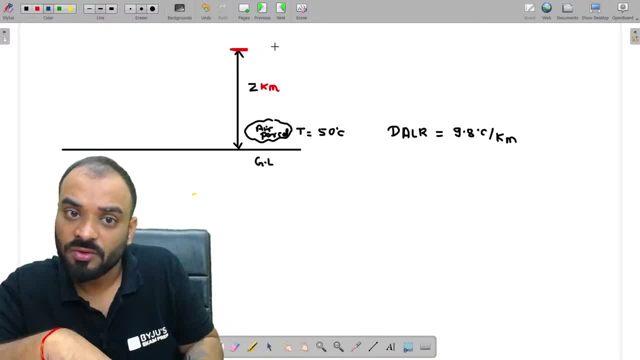 How much is the temperature at this particular level? How we can find it out very easy. So can I write here, guys, the initial temperature at the base is equal to 50 degree centigrade. Okay, Minus the rate is 9.8 degree centigrade per kilometer. 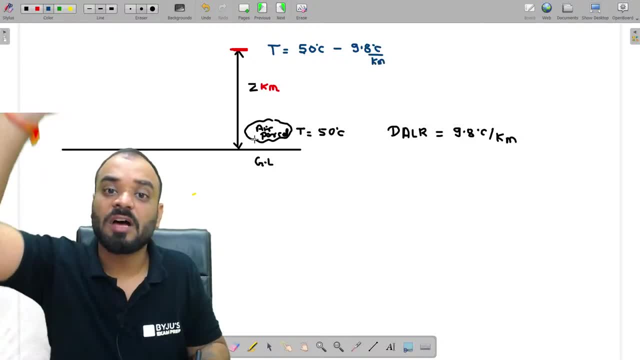 But we know that, guys, how much distance it has moved in upward direction. That is basically Z kilometer. So let's multiply it by Z kilometer. So this is the equation of temperature at a distance of Z kilometer from the ground level. 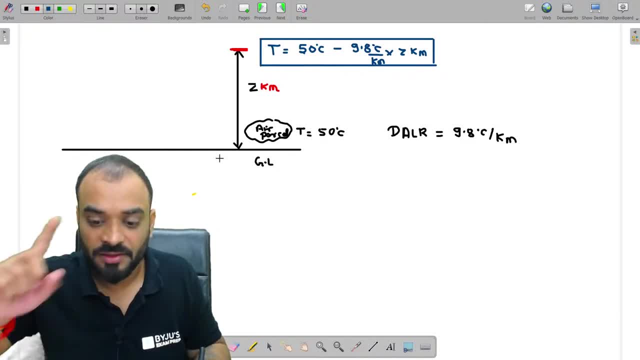 Okay, For the air parcel, for the air parcel. Now, if we talk about the surrounding air, they have already mentioned the relation for the surrounding air. guys, You can see here: for surrounding air, the relation is: Z is equal to minus 0.2 T plus. 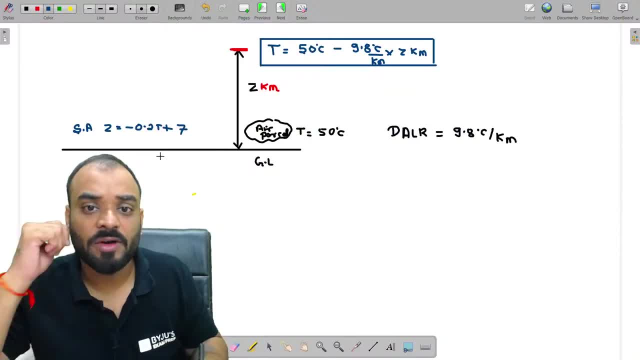 7. Correct Now, guys, can we find out after a distance of Z from the base or from the ground level, what should be the temperature of the surrounding air? Can we find out Right? We have to find this particular value. 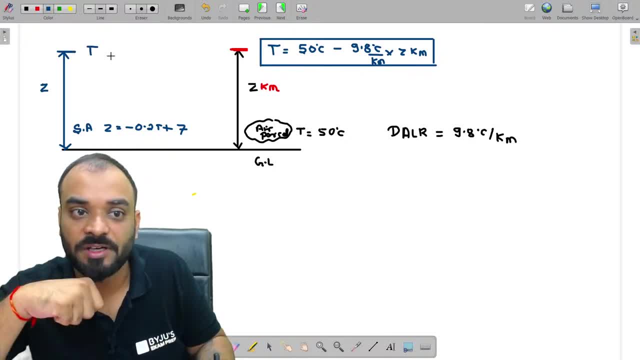 What is the temperature at this particular level? So can we find out. Just you have to resolve this particular equation. you will get it Okay. So can I write here, guys, this is nothing as basically Z minus 7 divided by Z minus. 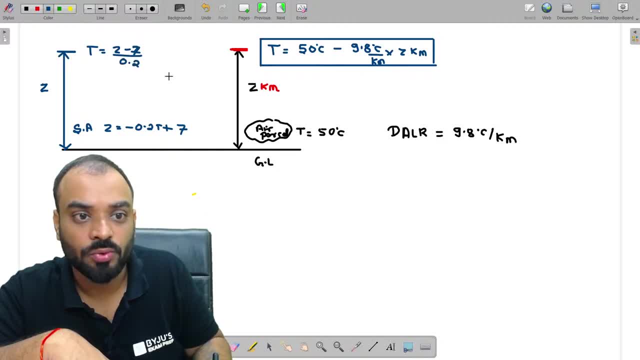 7 divided by 0.2.. Okay, So this should be the temperature at a distance of Z from the ground level for the surrounding air. Now, as for the question, we need to equate both of them. Okay, Okay. 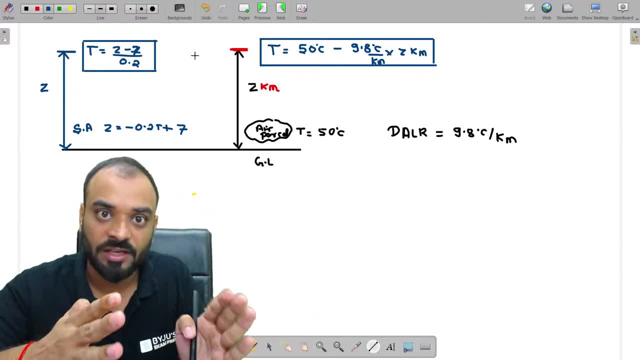 So that we will have the temperature of the surrounding air and the air parcel will be same. Okay, So you can see here, guys, if we equate it, what we will get as a result: Z minus 7, divided by 0.2, it should be equal to 50 minus 9.8 times of Z. 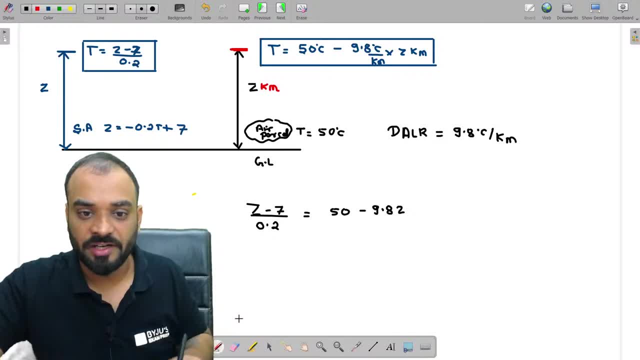 Okay, So let's resolve it. guys, How much we are getting? Kindly find it out and let me know the answer: Z minus 7.. Z minus 7 is equal to 50 into 0.2. That is equal to 10.. 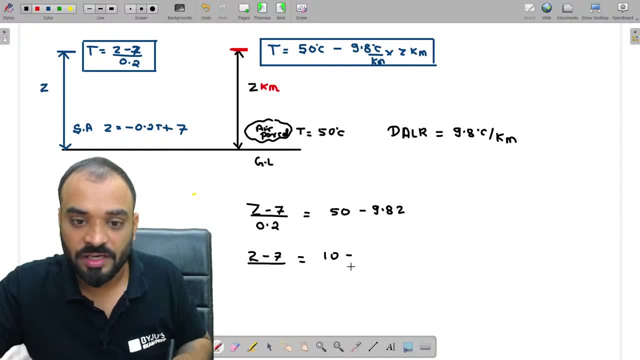 Okay, Then minus 9.8, multiplied by 0.2.. So we are getting a value of 1.96 Z. Okay, Let's shift it on the left hand side. So we are getting a value of 2.96 Z, and it should be equal to 17.. 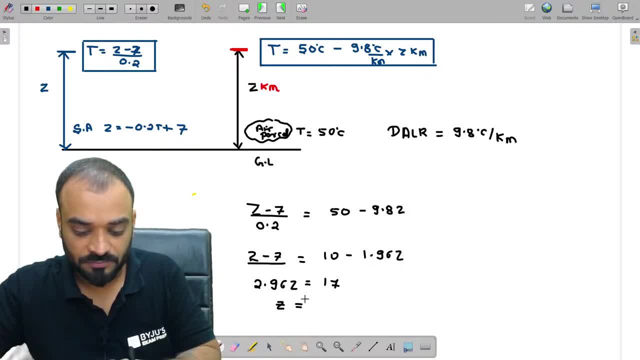 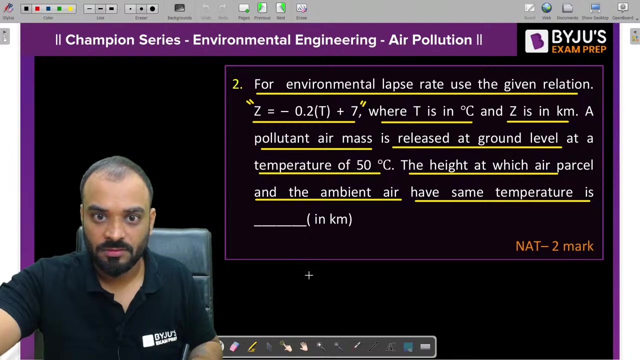 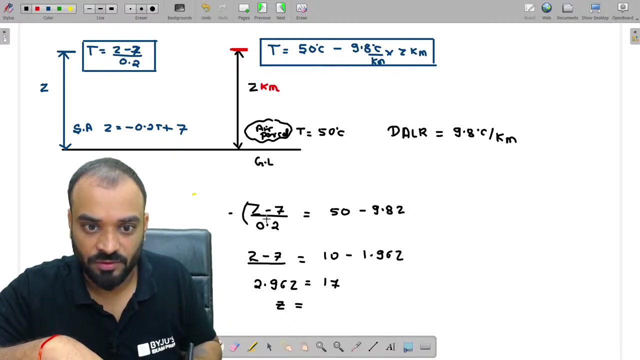 So what is the value of Z? Please let me know, guys. Okay, Okay, Okay, Okay. How much distance? Tell me guys. Okay, This equation is negative. Right, This equation is negative. Wait a second. This equation is negative. 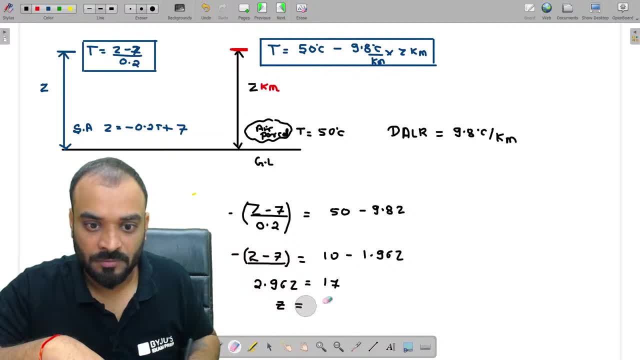 Okay, Tell me what is the value of Z guys? value of z guys in this particular case. so minus z plus 7, it is equal to 10 and this is minus 1.96 z. okay, let's shift it. so how much we are getting minus z plus 1.96 time of z, and it should be. 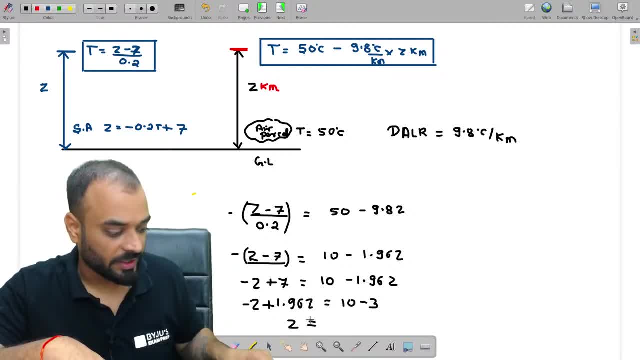 equal to 10 minus 3. so what is the value of z? please find it out, guys, how much we are getting. what should be the distance. anyone who can tell me? guys, it is coming around 3.125 kilometer, 3.125 kilometer. so at this particular distance, the temperature of surrounding air and the 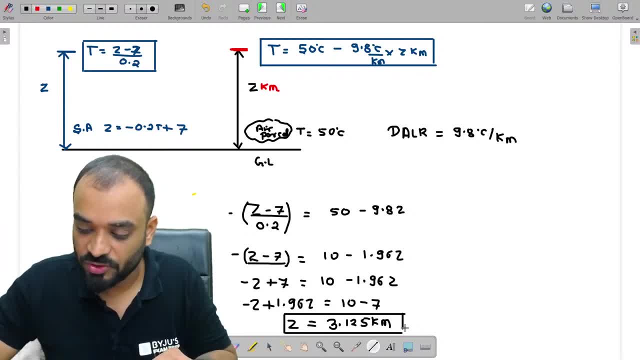 temperature of air parcel will become same. tell me, yes or no. the temperature of air parcel and the temperature of surrounding air will become same. you can find it out, guys, all also by putting this particular value in this particular case. so how much we are getting, minus z, plus 7. 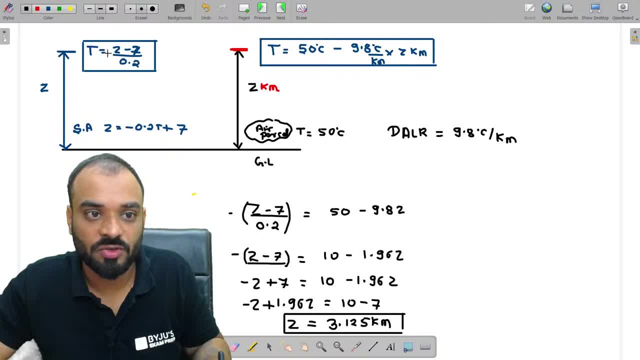 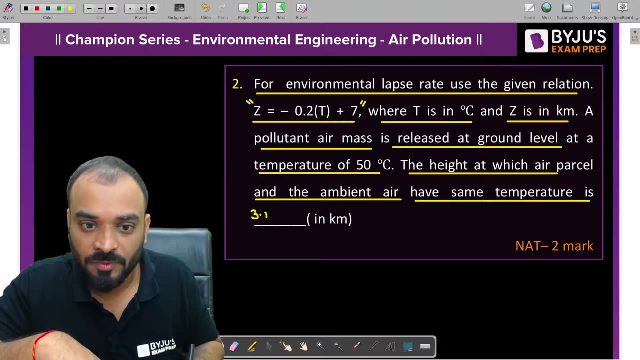 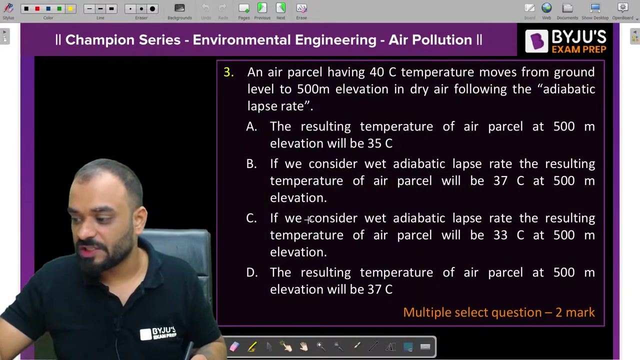 in this equation, and in this equation, you will get the same result. okay, you will get the same result. this should be negative. clear, crystal clear, guys, crystal clear. so the value is how much it is: 3.125 kilometer, 3.125 kilometer. okay, now let's solve the next question, guys, which is: 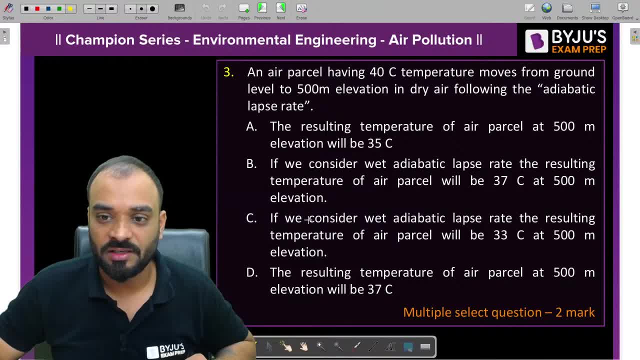 basically an msq question. another question, guys, which is a little bit you uh logical one and uh, no doubt, guys, such type of question you may also get in the examination. okay, so be careful while reading the problem first and then let me know the answer. okay, now what is given? 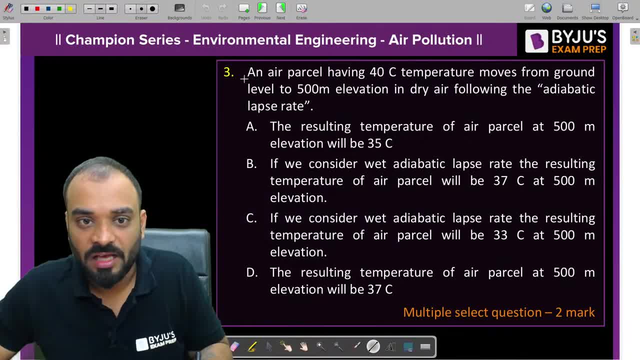 in the question. let's read it first. an air parcel having 40 degree centigrade temperature moves from ground to a level of 500 meter elevation in dry air following the adiabatic lapse rate. okay, let us suppose, guys, this is our ground level and at the same time we are getting minus z, plus 1.96. 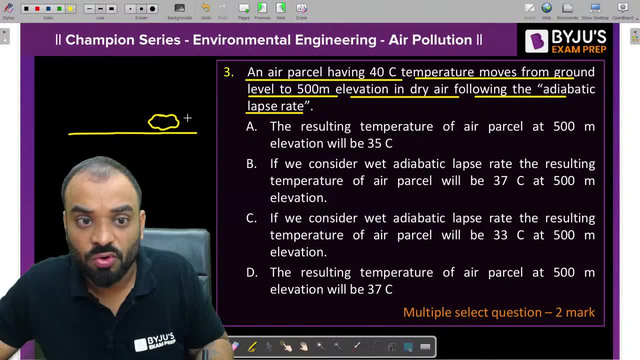 at this particular ground level, we are having an air parcel whose temperature is equal to how much, whose temperature is equal to 40 degree centigrade, and this particular air parcel is moving from the ground at a distance of 500 meter. okay, let us consider this. distance is equal to how much? this? 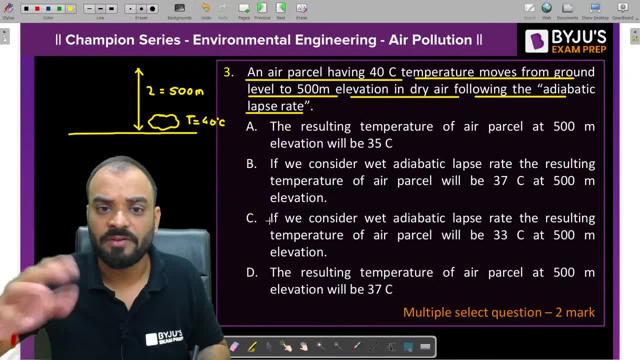 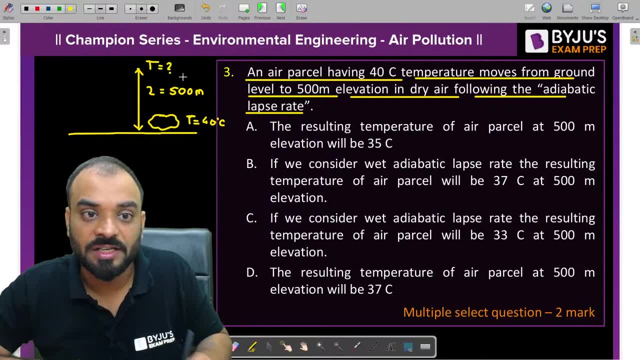 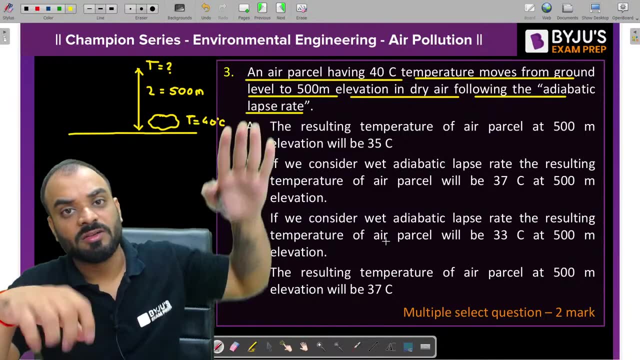 distance is equal to 500 meter, or you can call it as 0.5 kilometer. now our task is to find out the temperature at this particular level, what should be the temperature at this particular level? you know that, guys, whenever such type of air parcel is trying to move from the ground level in the upward direction, we have to prefer the dry. 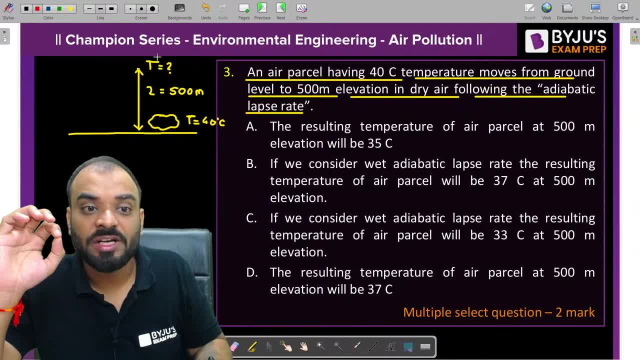 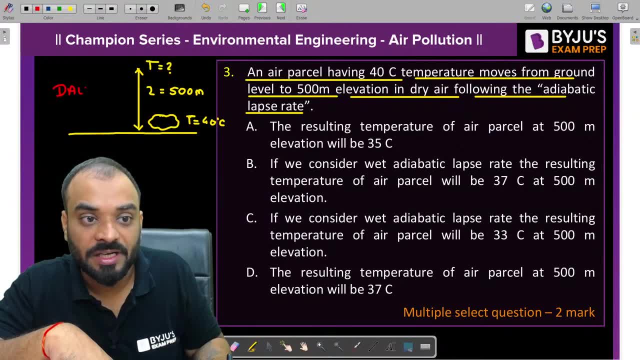 adiabatic lapse rate. okay, now we need to calculate this particular temperature by using dry adiabatic lapse rate. now tell me, guys, what is the value of dry adiabatic lapse rate? you know that, guys. generally it is 9.8 degrees centigrade per kilometer clear. now can we calculate the. 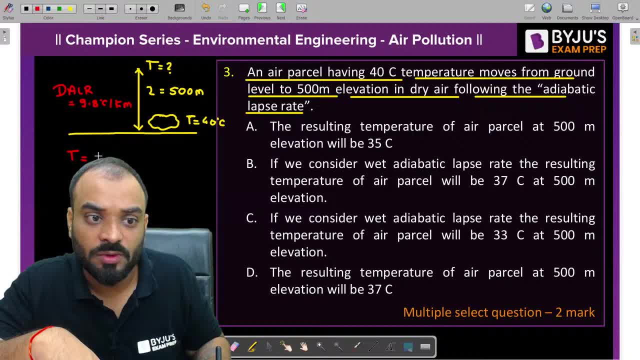 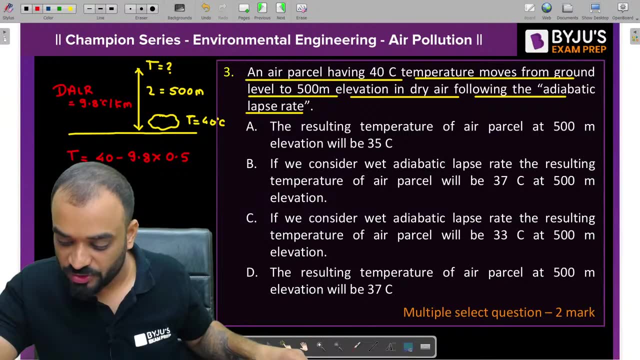 temperature at this level. yes, so let's calculate it. t is equal to how much? it is 40 degree at the base, or you can call it as: at the ground level, minus, the rate is 9.8. multiply by how much the distance is 0.5. okay, so let's solve it. guys, how much we are getting chance? 0.0065, no, 40 minus 40. 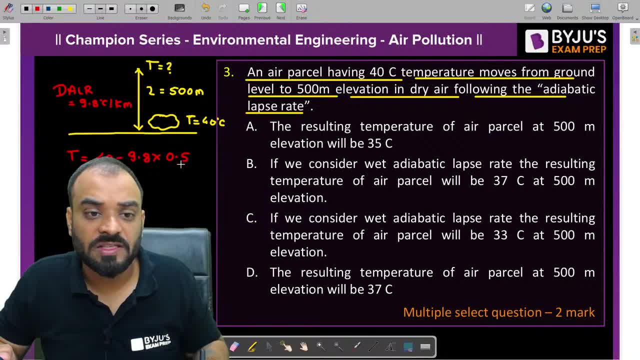 minus nine point eight chance. listen carefully, guys. you need to put this particular value of this distance in terms of kilometer, not in terms of meter. okay, so how much? we are getting 35.1, 35.1 degree centigrade, which is also equal to 35 degree centigrade. we can call it as: 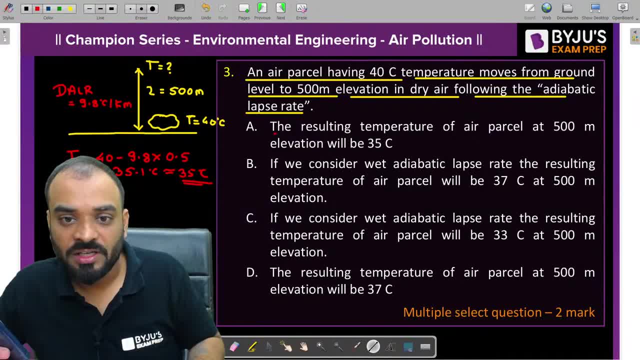 35 degree centigrade also right. so let's read the option first. the resulting temperature of air parcel at 500 meter elevation will be 35 degree centigrade. yes, it is correct or wrong? yes, it is correct. a is the correct answer, yes or no? 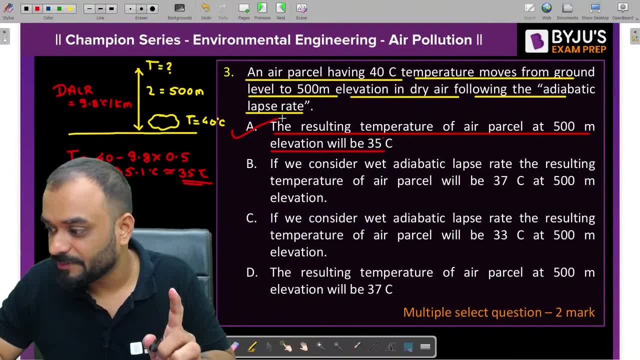 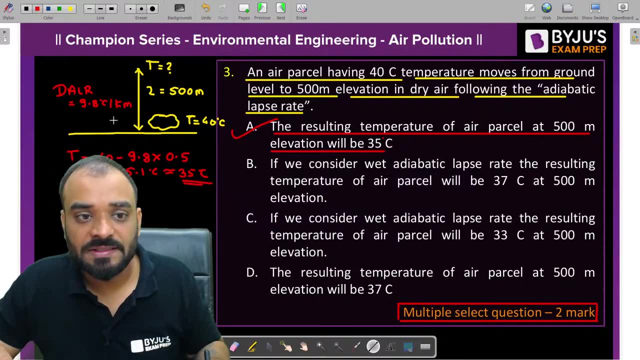 guys, a is the correct answer, yes or no? tell me, a is the correct one, because this one is msq. we need to find out the multiple option which can be correct over here. very nice, now let's read the next one. now, guys, such type of condition in which we have solved the problem, that is basically the 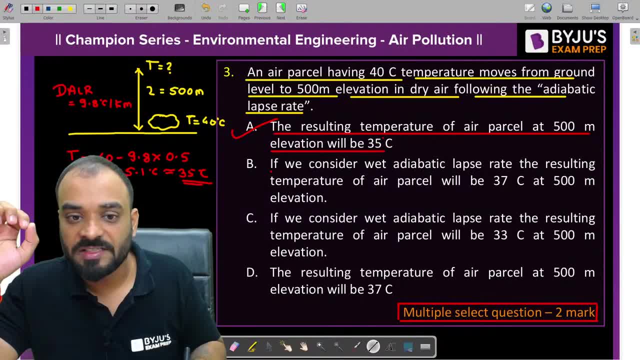 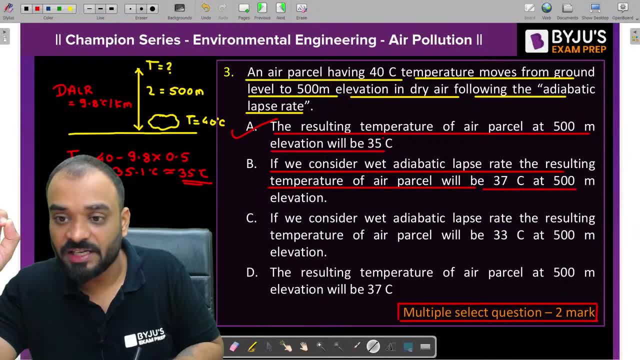 dry adiabatic condition. but let us suppose if we consider the wet adiabatic lapse rate, the resulting temperature of air parcel will be 37 degree centigrade at 500 degree, 500 meter elevation. now, guys, when we have the wet adiabatic lapse rate, wet adiabatic lapse rate. 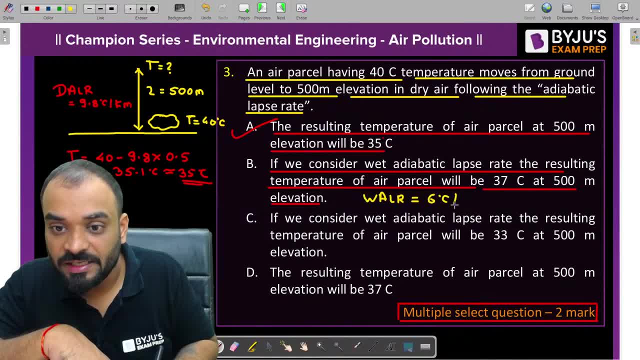 so wet adiabatic lapse rate is equal to 6 degree centigrade per kilometer. this should be the rate. can we calculate the temperature guys again at this particular level? when we are considering, in place of dry adiabatic lapse rate, we have to consider wet one. okay, let's do it. 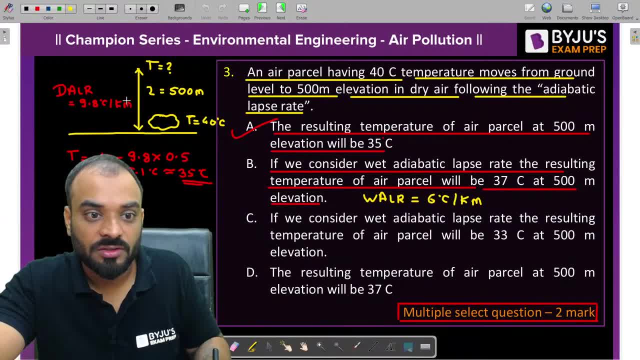 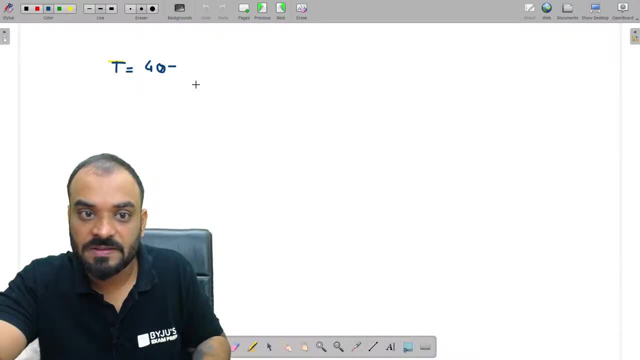 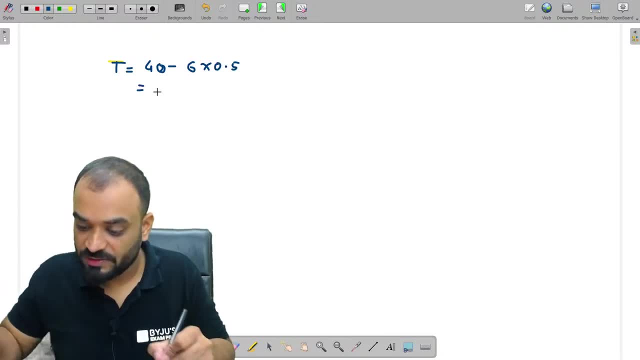 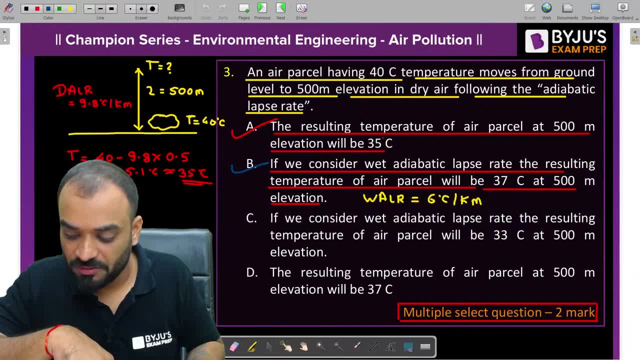 yes, prathmesh, this option can also be correct. b is also correct because we are getting 37 degree centigrade as answer when we are considering wet adiabatic lapse rate. okay, b is also correct. now let's read the next one. if we consider wet adiabatic lapse rate, the resulting temperature. 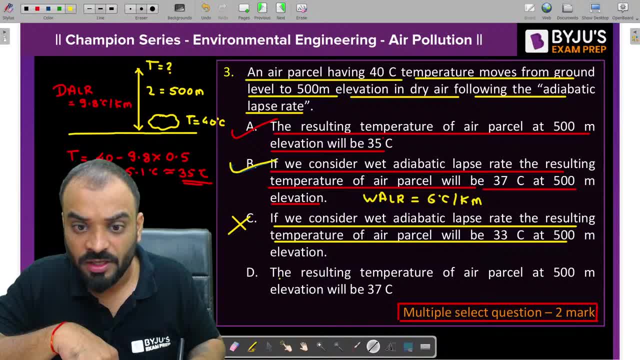 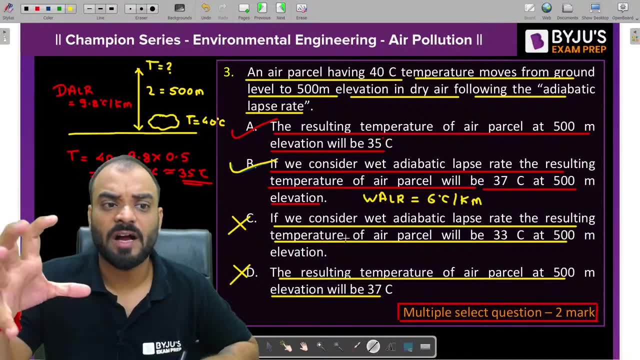 of air parcel will be 30 degree centigrade. no, it is wrong. the resulting temperature of air parcel: no, it is also wrong why? because, guys, in general we have to consider dry one or dry adiabatic lapse. we are getting the temperature as 35 degree centigrade, not the 37 one. okay, that's why c. 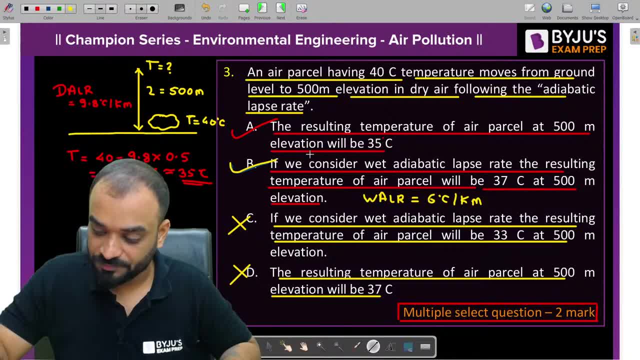 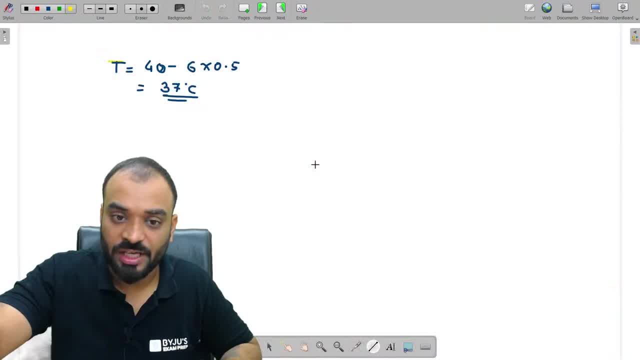 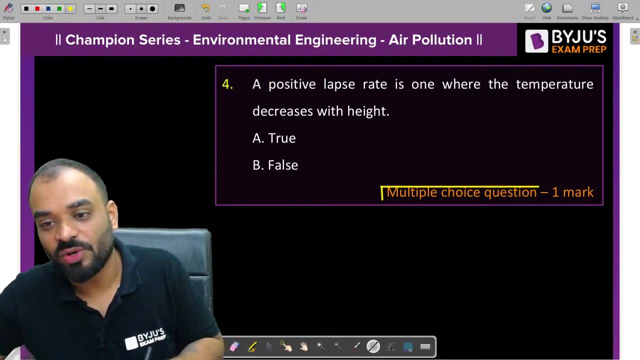 and d option are wrong. only a and b are the correct one. very nice, prathmesh, very nice, okay, so let's move to the next question, guys. let's move to the next question now, guys. this is a mcq type question, but guys, uh, basically it is a true and false question. 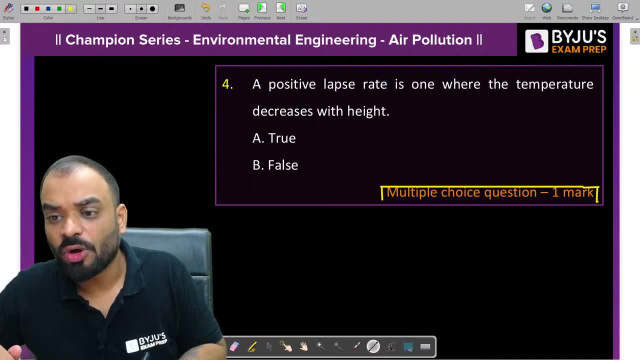 okay and such type of question. you may get a with a four option also in your examination. but let me know, guys, if you have any questions, please let me know in the comment section. so, guys, which one is the correct answer over here, whether it is a or b? 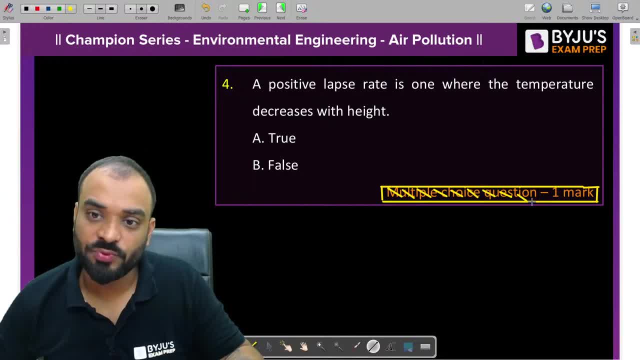 whether it is a or b. a positive lapse rate is one where the temperature decreases with height. a positive lapse rate is one where the temperature decreases with height. this statement is true or false? this statement is true or false? tell me guys quickly. a positive lapse rate is one where the temperature decreases with height. 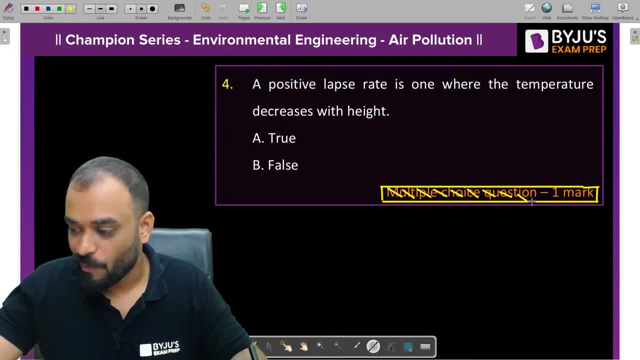 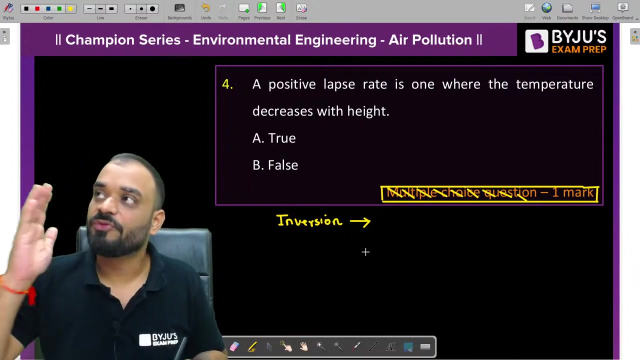 confused. okay, have you heard about the inversion condition? inversion condition, inversion condition, true, prathmesh? very nice, true guys. what is basically inversion? let me explain what is basically inversion. inversion is nothing, as in this particular scenario, what will happen? the rate of change of temperature with respect to height will become positive. that means if you move. 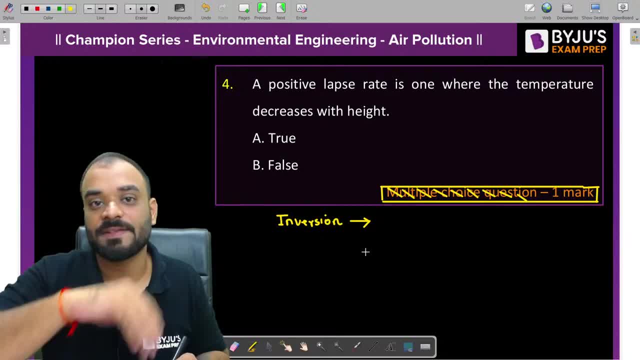 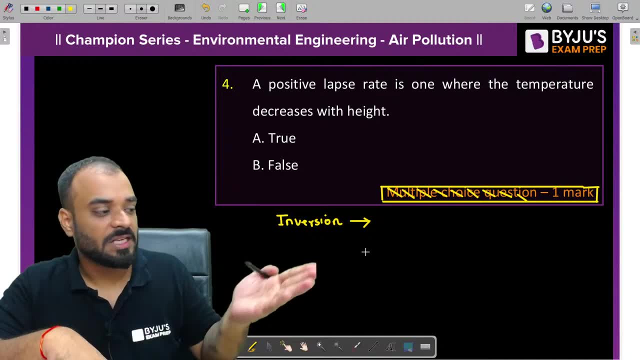 in upward direction. the temperature is also increasing. that is not decreasing, that is not decreasing. but, in general, what will happen, guys? in general, what will happen, basically, when we are trying to move in upward direction, so our temperature is trying to reduce- right, our temperature is trying to reduce- and such type of- uh uh general, uh, general change in temperature? 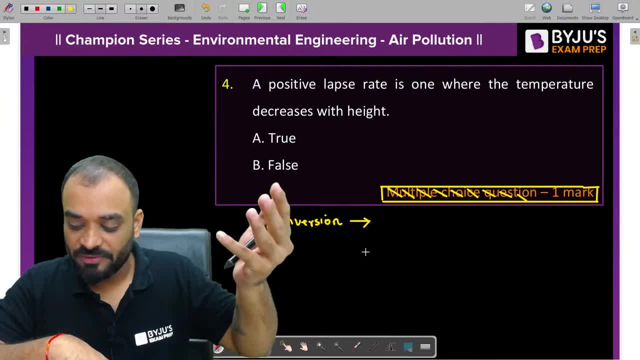 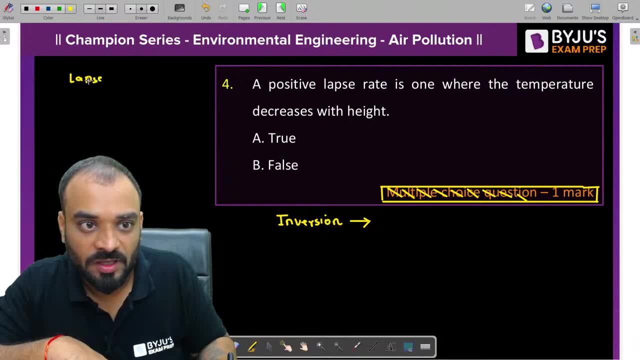 with respect to height is nothing as our lapse rate. but, guys, if you are having the positive lapse rate, positive lapse rate means what? let me write here in general what will happen. let me show you that. then we will discuss. what is this condition exactly? let us suppose this is a graph. 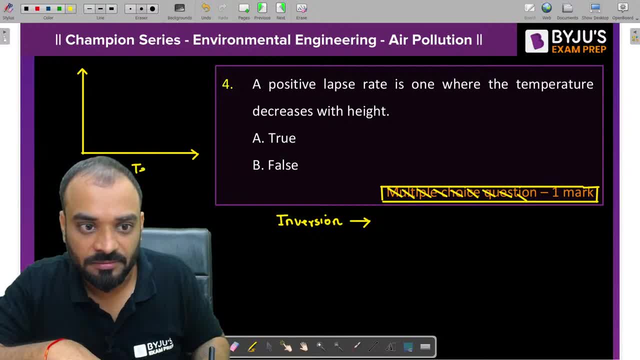 between the temperature and the height. right, let us consider right now. at the ground level, the temperature is t1. okay, when we are trying to move in upward direction, so our temperature is trying to reduce and let us suppose we have reach at a distance of z2. okay, let us consider this distance. 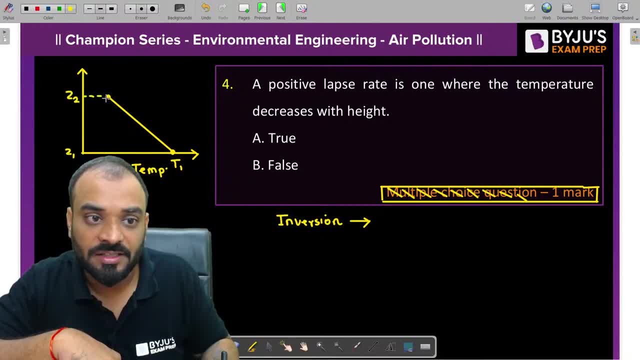 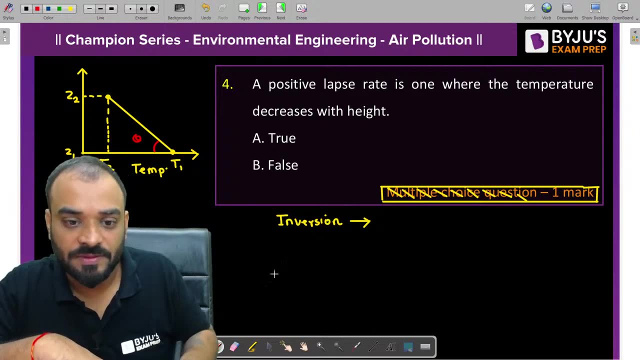 is z2 and this distance is z1, okay, and the temperature at this particular level is equal to what? that is, basically t2. now, what is our task? our task is to find out this particular uh slope. okay, what is this slope? this is nothing as our lapse rate in general. now you can see here, guys, sorry, we have to find this one. 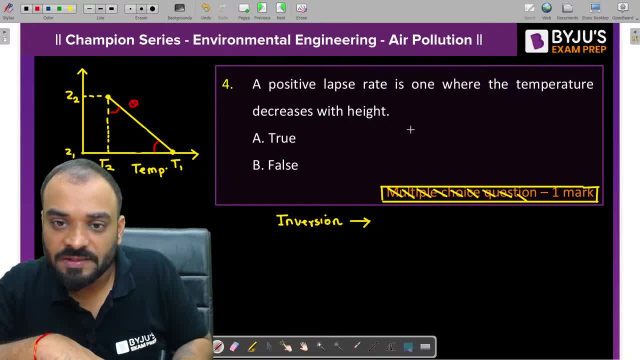 this particular slope. okay, now you can see here, guys, can i write here the lapse rate? lapse rate is equal to what this is in general. now tell me, guys, what is this particular lapse rate? okay, so we can see here. initially, the temperature is t1, which is higher, okay, minus t2. okay, now we can. 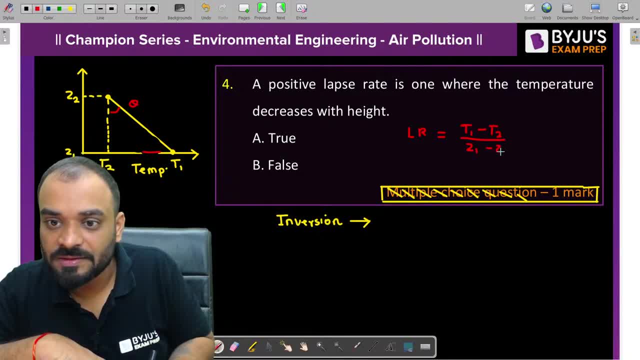 see here, guys, the distance z1 minus z2. but we know that, guys, z1 value is lesser than z2, so definitely we are getting a negative value at the base. so can i write here, guys: this particular value will become minus of t1 minus t2, divided by z2 minus z1. 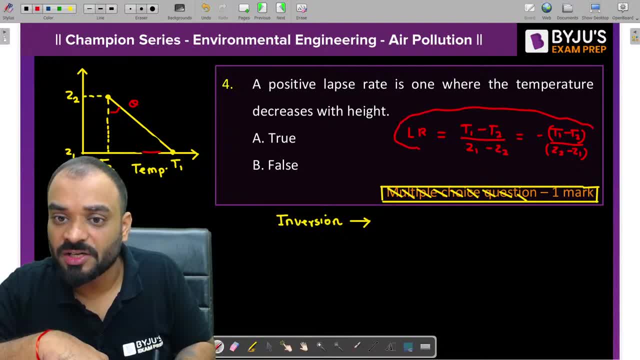 so can i say that, guys, in general our rate of temperature, rate of change of temperature with respect to height, is negative in general. but, guys, if you are having a positive value, if you are getting a positive value, that means if this particular change is positive, how we can represent. 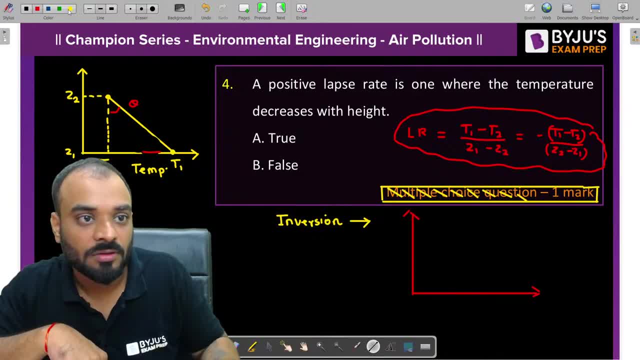 it. let me show you that also. so, again, this is our height above the ground and this is basically temperature in degrees centigrade. now let us suppose, guys, our graph is like this and initially the temperature is t1 and the distance is z2, and this is our height above the ground and this is 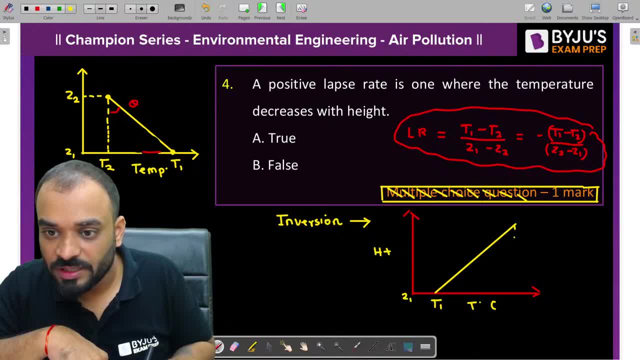 z1. and let us suppose at this particular level, the temperature is t2 and the height is z2. now, guys, we need to find this particular slope. okay, now, how much it is. can i write here, guys? the lapse rate is equal to t1 minus t2, or what we can write here, guys, let's write t2 minus t1, because we know. 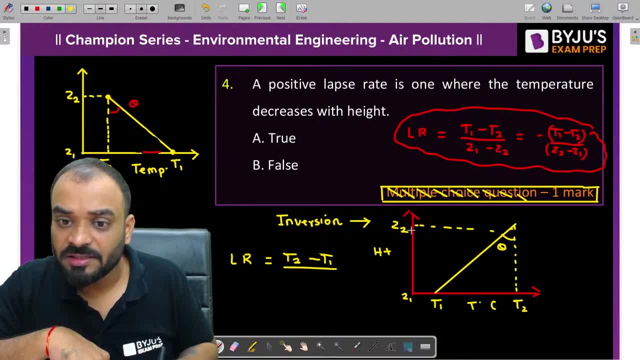 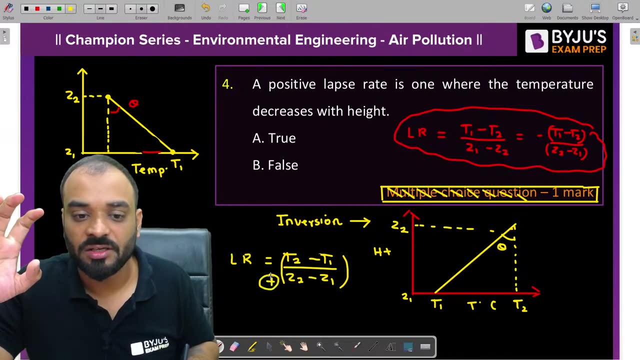 that t2 is greater, so t2 minus t1. and can we write z2 minus z1, z2 minus z1? now tell me guys, the numerator value and the denominator value. both the values are positive in nature, so ultimately you will get a positive result at the last. now, such type of rate. 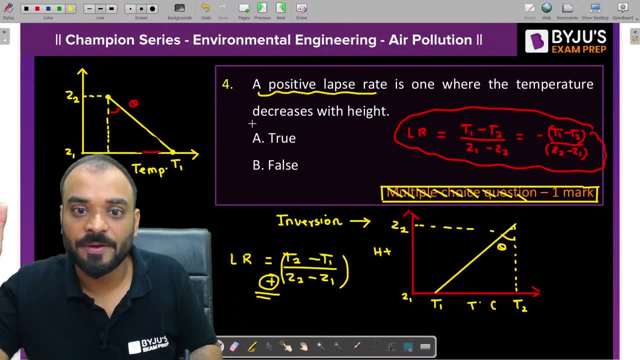 is known as positive lapse rate, which is where the, where the temperature decreases with respect to height. now let me explain one more thing over here, guys. this particular condition where you are getting the positive result, it is known as negative lapse rate. negative lapse rate, and this general one. this general one is known as positive lapse rate. 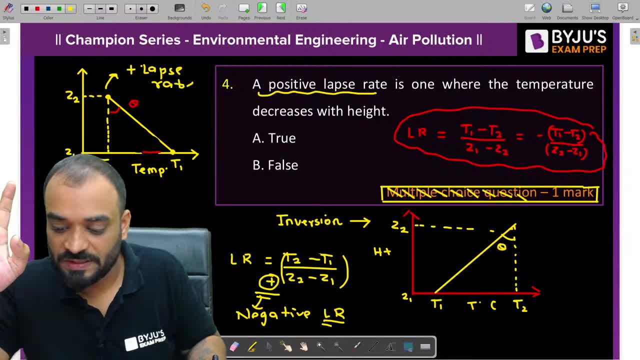 which is a standard condition. right, which is a standard condition? okay. so in general, we know that, guys, our temperature will decrease with respect to height. that's why this statement is true and this particular statement is true. why? because this is a positive lapse rate in general, but if we talk about the negative or inversion condition, which is nothing as our negative lapse, 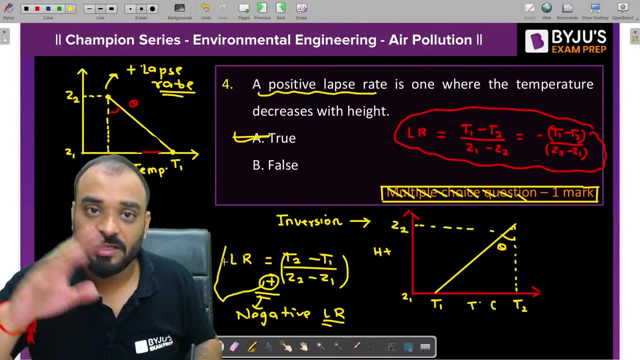 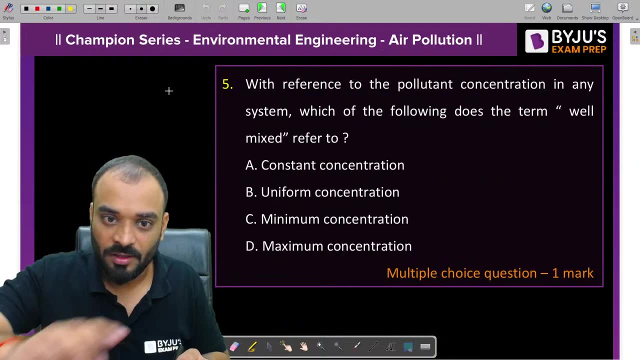 rate in general, right? in case of negative lapse rate, you are getting a positive result, but in case of positive lapse rate, you are getting a negative result, right? that is the conclusion of the discussion. next question, guys, in front of you. next question in front of you. next question in front of you, with. 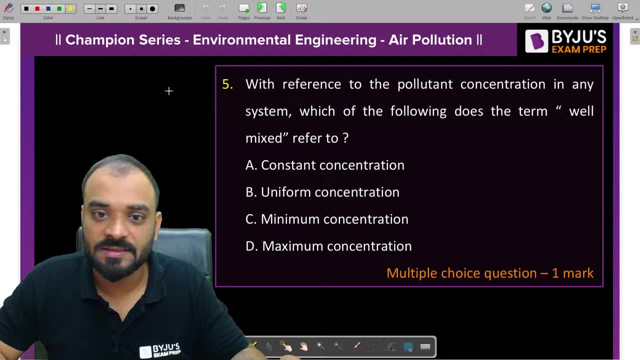 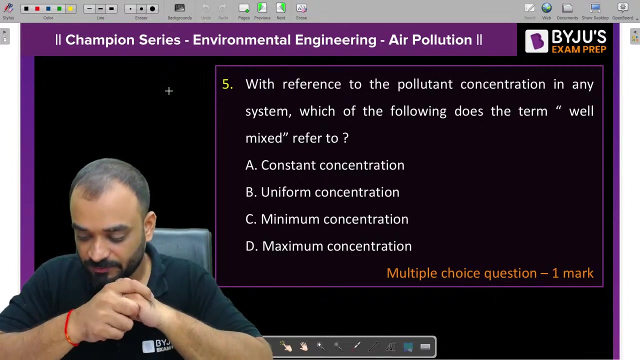 reference to the pollutant concentration in any system. which of the following does the term well mixed refer to you, guys, what you mean by well mixed? what do you mean by well mix? tell me, guys, one more question in front of you. what do you mean by well mixed system? it is c, minimum concentration, no nps and- sorry, nsp. 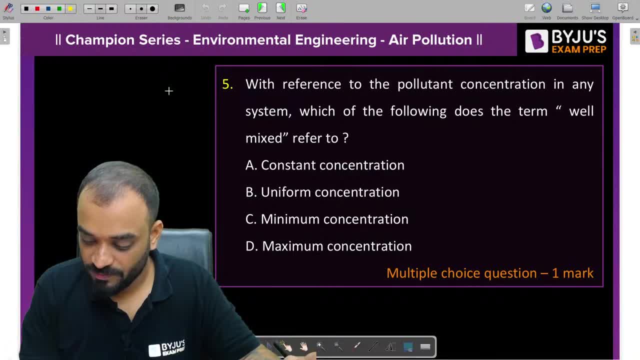 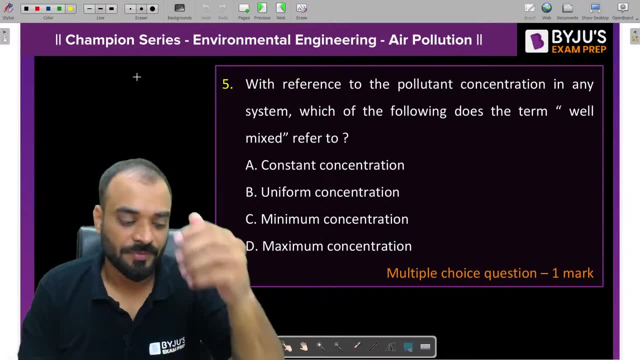 guys. well, mix is what? let us suppose if you have a glass of water, in that glass of water, if i add one spoon of sugar and try to mix it very well, right? so that means whatever sugar you have added, that should be present in each and every drop of water. that means our concentration should be. 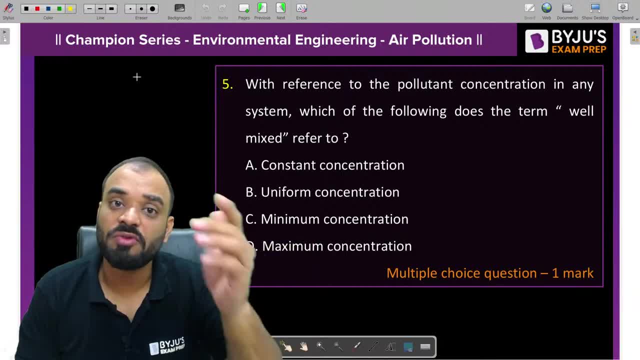 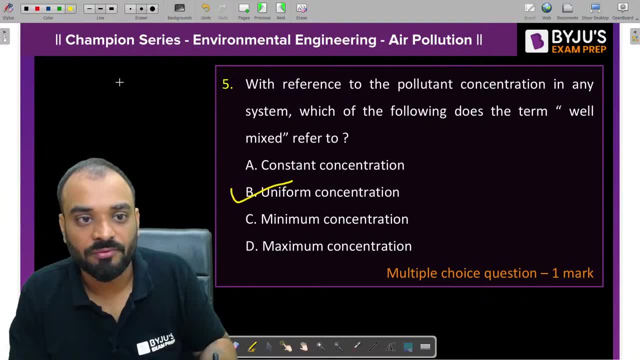 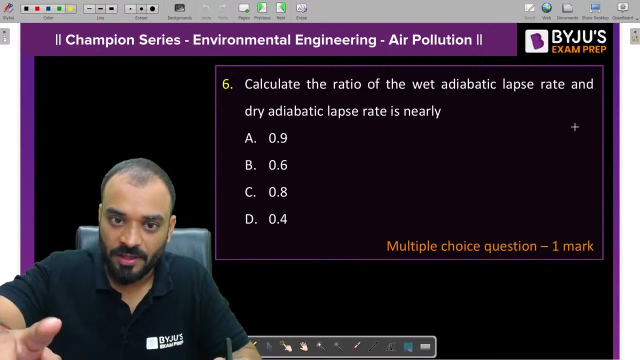 uniform right. so well, mixed with nothing, as it is a uniform concentration of the pollutant. that's why, guys, the b is the correct answer for the problem. b is the correct answer for the problem. well, mixes, uniform concentration. basically clear, uniform concentration. uniform concentration, clear, okay question in front of you guys. again one more question: mcq type problem. 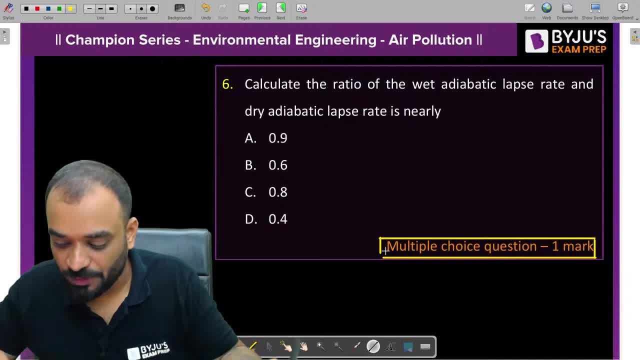 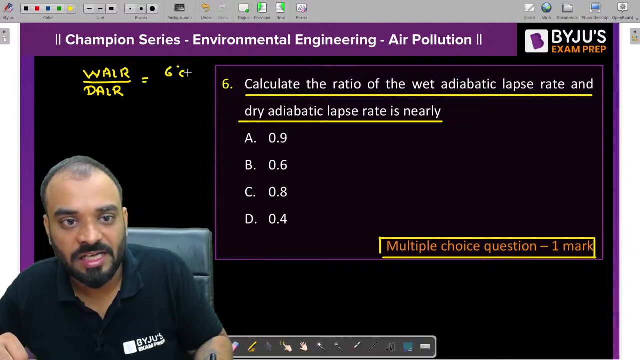 mcq type problem. now what you need to do, guys over here, you need to calculate the ratio of wet adiabatic lapse rate and the dry adiabatic lapse rate. the ratio of wet adiabatic lapse rate upon dry adiabatic lapse rate: what is the ratio of it, guys? you know that wet adiabatic lapse rate is. 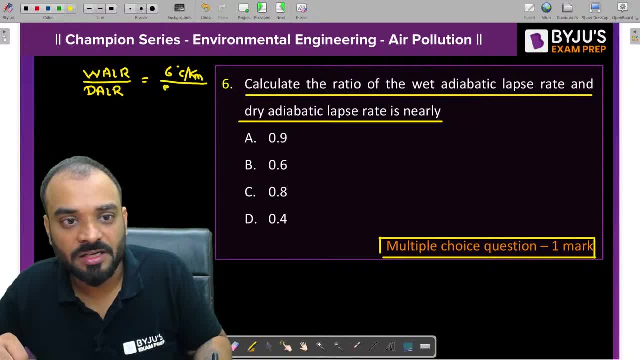 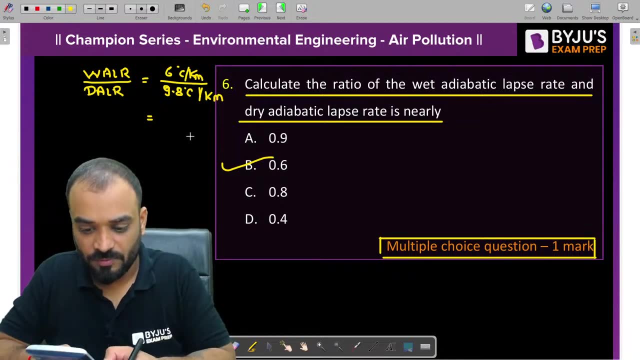 six degrees centigrade centigrade per kilometer, and the dry one is 9.8 degree centigrade per kilometer. now tell me guys, what is this ratio? prathmesh b: 0.6. very nice, it is coming around. how much, right? 0.61 something. 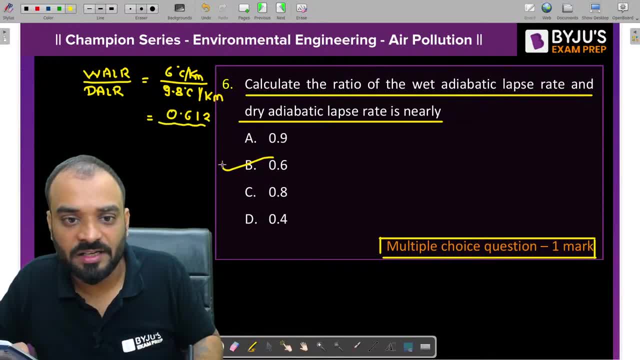 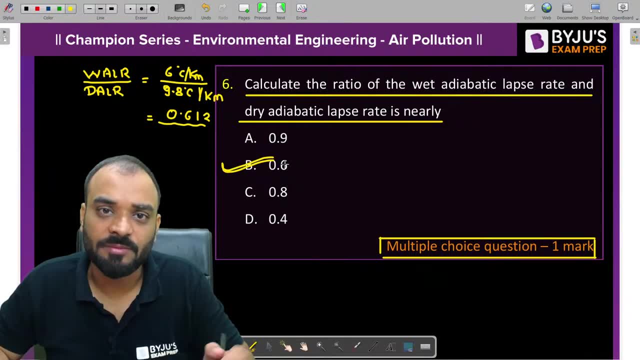 right, 0.612 right. so we can say that b is the correct answer. but, guys, what happened? let me explain one more point over here. what happened? uh, sometime, sometime, uh, in some of the book they are also referring the dry adiabatic lapse rate as a 10 degree centigrade per kilometer. 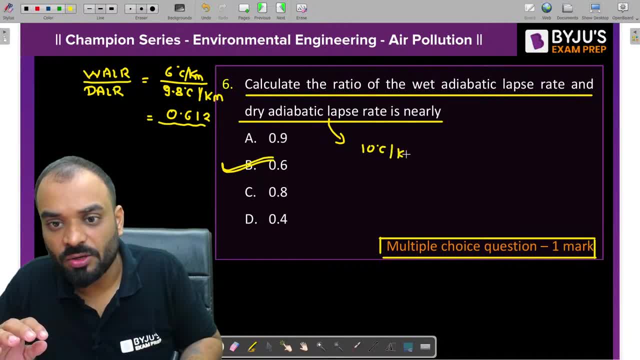 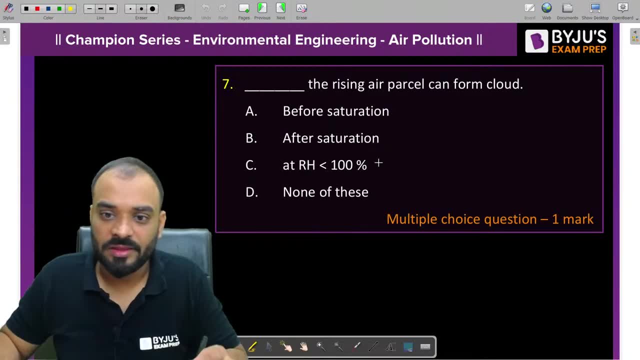 right, so you can use this particular parameter also. either you can use 9.8 or 10 also, there is no issue. okay, b is the correct answer for the problem. next question, guys in front of you, mcq type problem: one mark dash, the rising air parcel can form cloud. 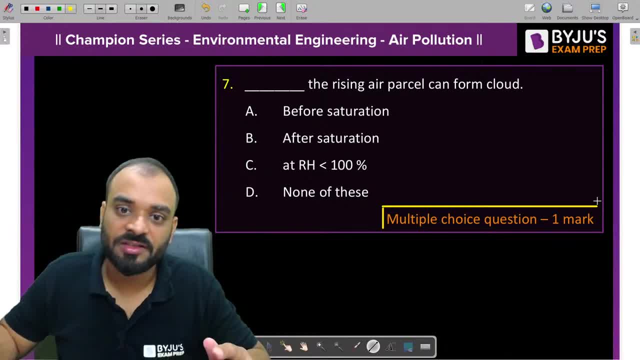 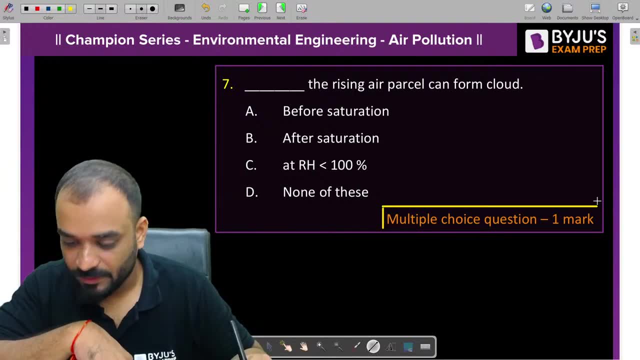 dash. the rising air parcel can form cloud. tell me, guys, what will be the answer for this particular problem? what will be the answer for this particular problem? a shian's, a before saturation? no, let me explain, guys. let us suppose this is your ground level and from the ground level we are releasing some air parcel, air parcel right now. what happened, guys? 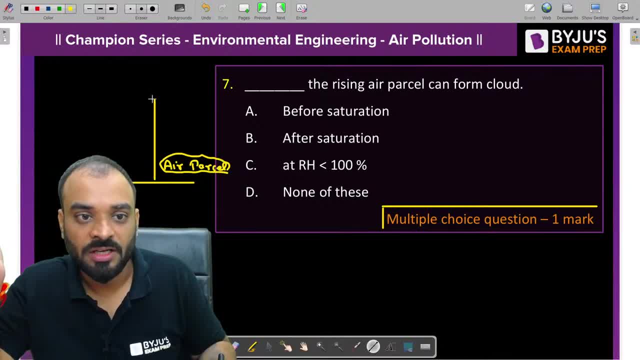 when this particular air parcel is released. from the ground level we are releasing some air parcel and from the ground level we are releasing some air parcel is trying to move in upward direction. it is trying to cool down itself by using a dry adiabatic lapse. 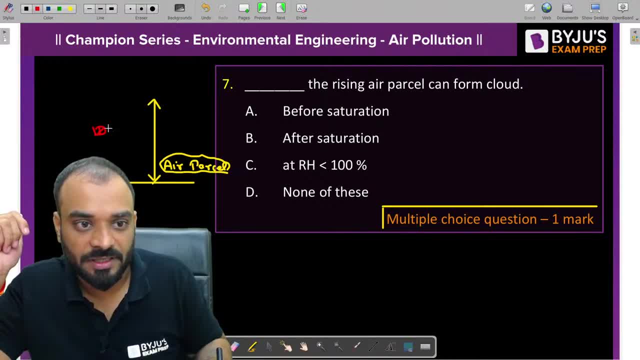 rate right. dry adiabatic lapse rate. it is trying to cool down itself by using a dry adiabatic lapse rate. now, after reaching a zone where the cloud is present, now, after reaching a zone where the cloud is present, what will happen? basically, this air parcel. let us suppose we will reach over here. 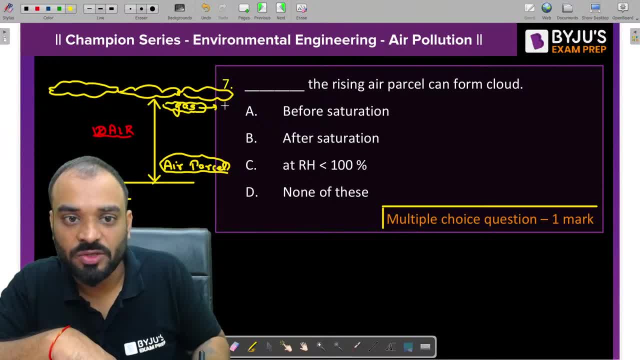 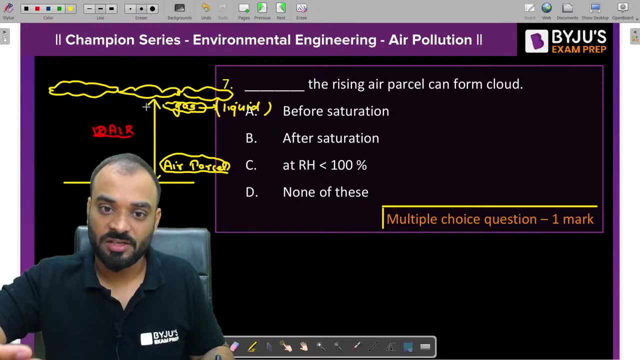 which is a basically a gaseous one. now this gaseous one is trying to convert it into, into a liquid one right now. whatever some particles are there, guys, they are trying to convert it in terms of liquid. so basically, it is trying to form a cloud when it is trying to get a saturation condition right? 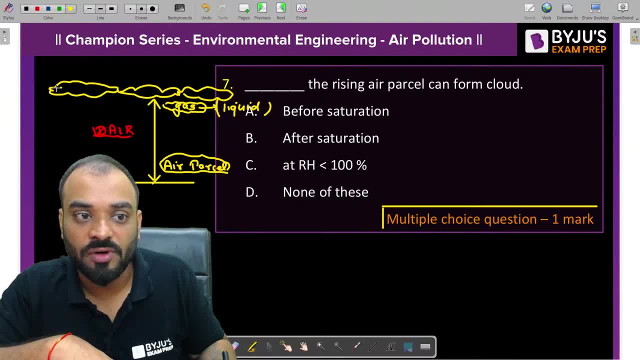 after saturation condition. so after this particular level of cloud, whatever rate of change of temperature of air parcel is there, that is to be considered as a wet adiabatic lapse rate, and wet adiabatic lapse rate is considered when your air parcel is hundred percent saturated. 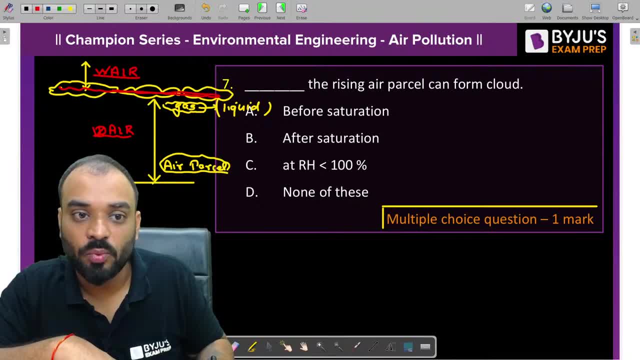 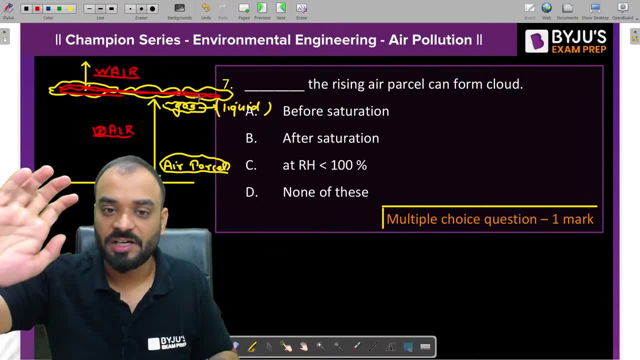 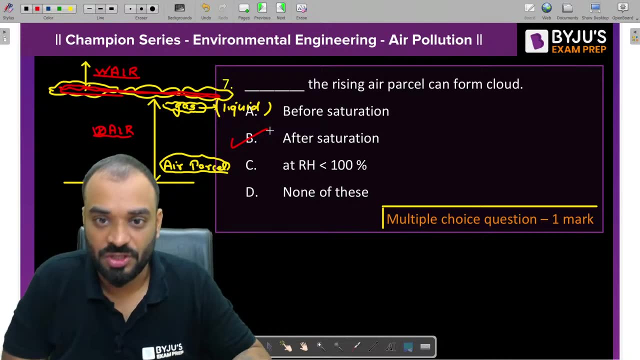 right. so at this particular level we can say that, guys, where the cloud is there, your air parcel will try to form a cloud after the saturation condition is there. that's why b is the correct answer for the problem, not a before saturation. it is after saturation. after saturation- clear next question, guys. 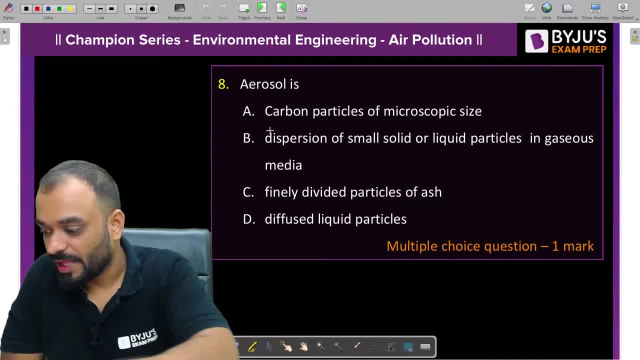 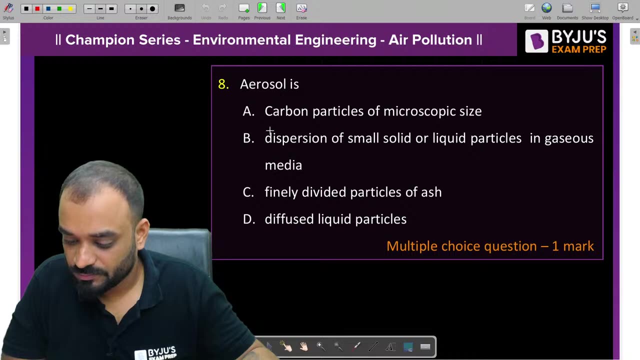 next question: aerosol is what. what is aerosol? what is aerosol? what is aerosol? tell me, guys, anyone who can tell me the answer, what is aerosol? basically, guys, aerosol is nothing, as it is the uh particle whose size is less than a molecule. 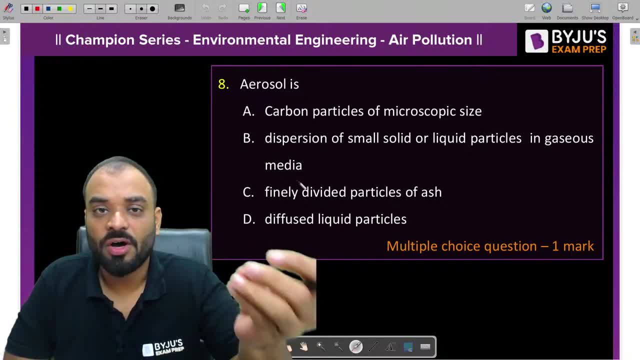 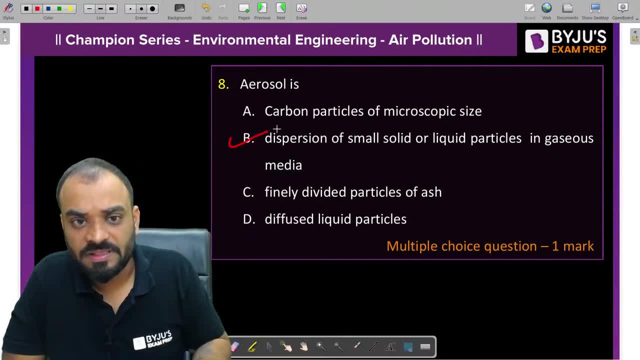 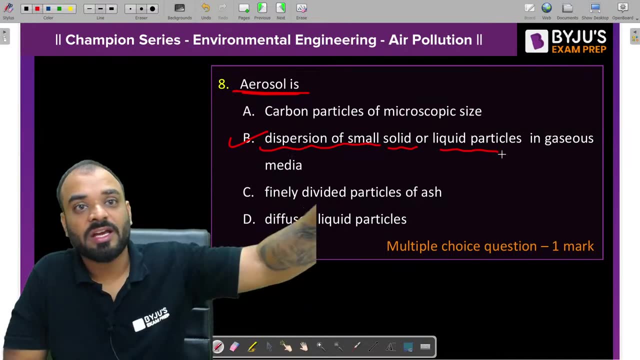 and it is in the form of solid or in a liquid form which is present in a gaseous media, and such type of particle is known as, basically, aerosol. okay, it is the dispersion of small solids or liquid particle which remain in suspension in the gaseous medium or in the air. that's why b is the 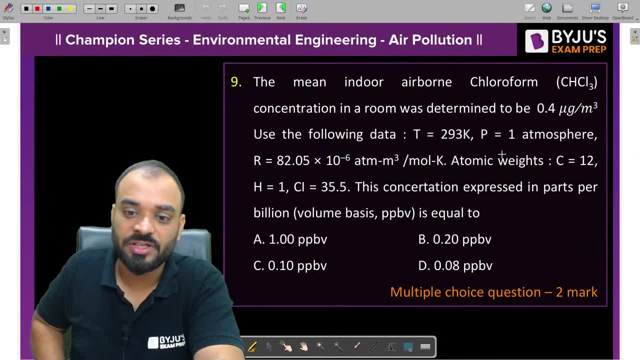 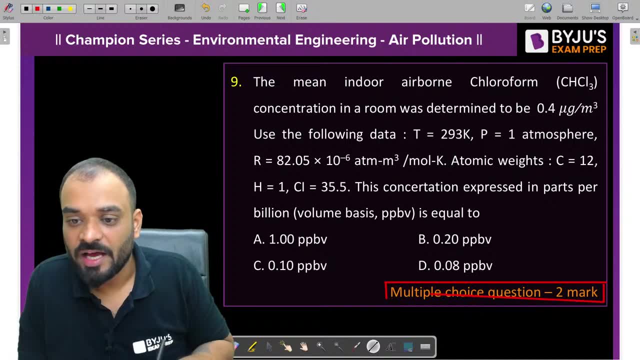 correct answer for the problem. now, guys, the last question in front of you, which is basically based upon the unit conversion, and it is a mcq type problem in which we will discuss how to convert the unit of air pollutant. okay, now let's read the question first, then we'll. 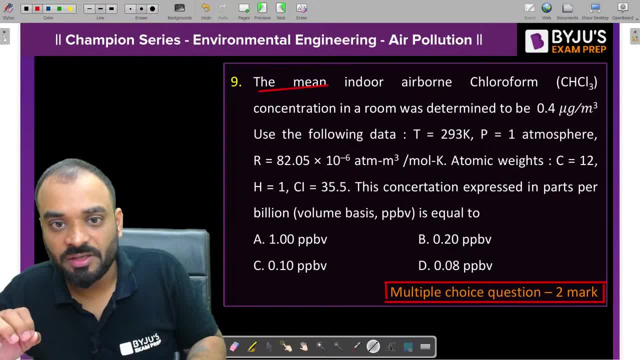 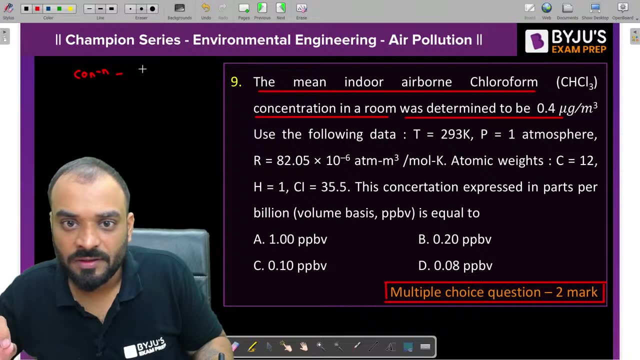 solve it now. what is given in the problem? let's understand the mean: indoor air bond coliform right concentration in a room was determined to be is equal to this right. so they have given the concentration, concentration of chloroform which is present inside a room and that 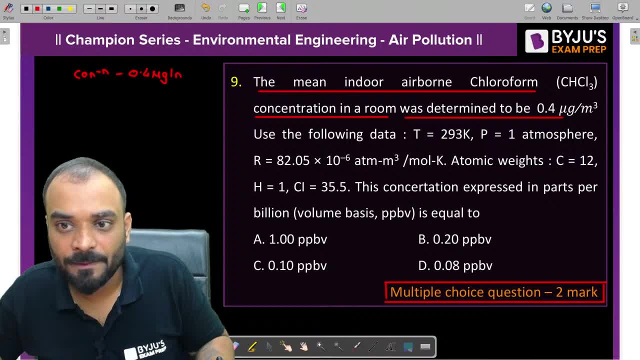 is equal to 0.4 microgram per meter cube. okay, now you need to use the data. the temperature is equal to how much? it is 293 kelvin, okay, and the pressure is equal to 180 m. okay. and the value of r is also mentioned, which is 82.05. 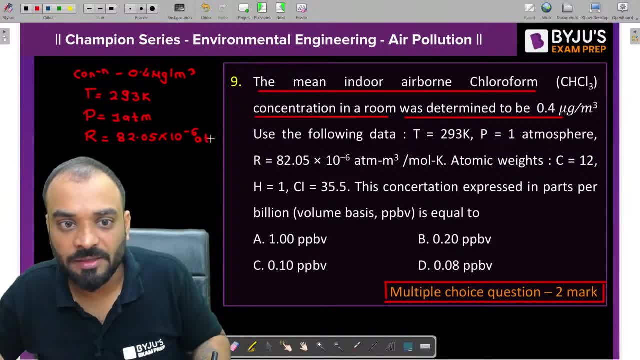 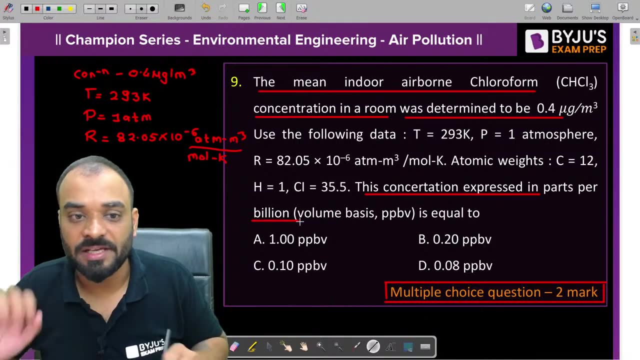 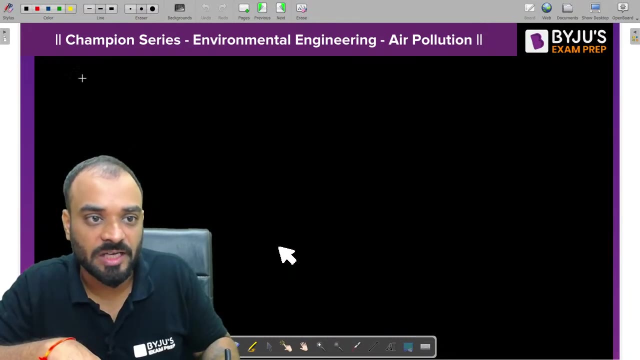 into 10 rest power minus 6 ATM meter cube per mole per Kelvin. okay, now our task is to find out the concentration which should be expressed in terms of part per billion. part per billion, right. so let's calculate it how much it is. so what we will do. first, guys, let me show you the relation. 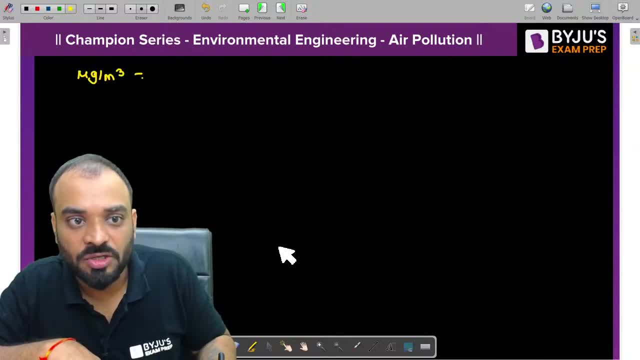 one relation is there which we have to use: microgram per meter cube should be is equal to how much it should be is equal to ppn. part per million multiply by 10. rest power 3 multiplied by molecular weight divided by volume, which is in terms of liter per mole. 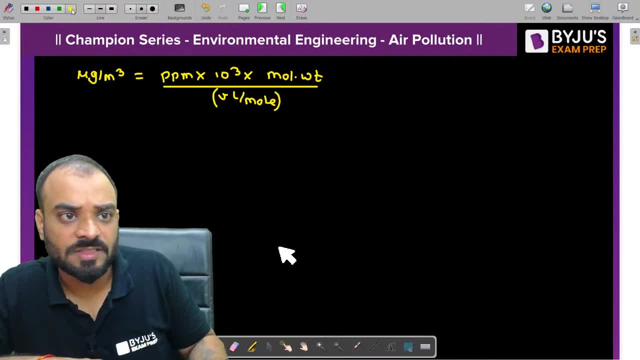 liter per mole. mean times it moves by how muchility term which is normal. r and r is equal to the number of millimeter square. so Пp, You will, by R, mars, dip some r in pp. right, this is bp, I, dp and pd, pp. Bp is equal to this. 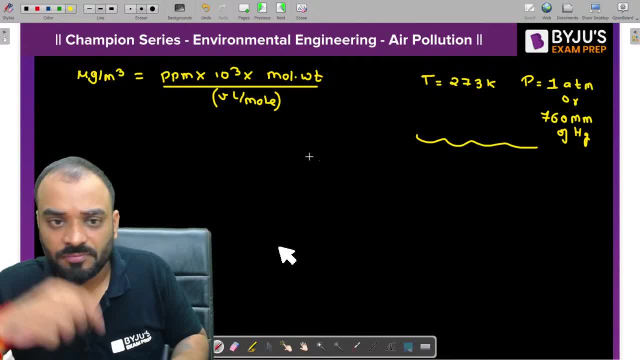 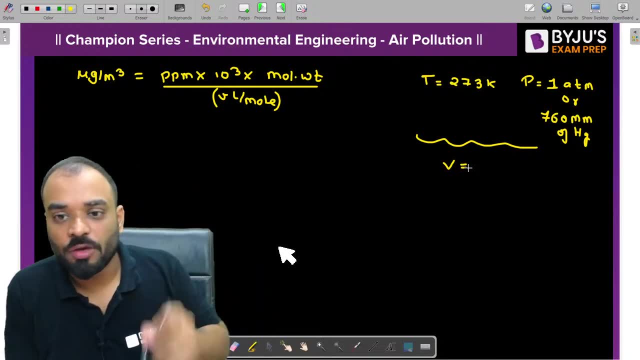 now, guys, we are having some standard value. when the temperature is 273 kelvin and pressure is equal to mole of any air pollutant will occupy 22.4 liter of air. right, right, okay. but we know that, guys, in such condition we are having a different temperature, but the pressure is. 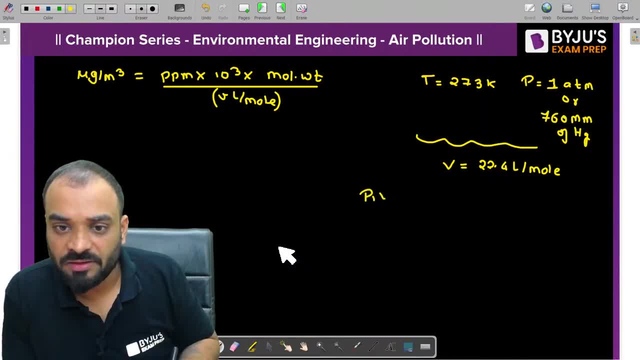 same. okay, so we can use a relation which is basically P1, V1 upon T1, and it should be equal to P2, V2 upon T2. now, at this particular condition, let us consider: temperature is T1, P1 and this is V1. we need to find out the V2 value, so this value is equal to how much P1 is equal. 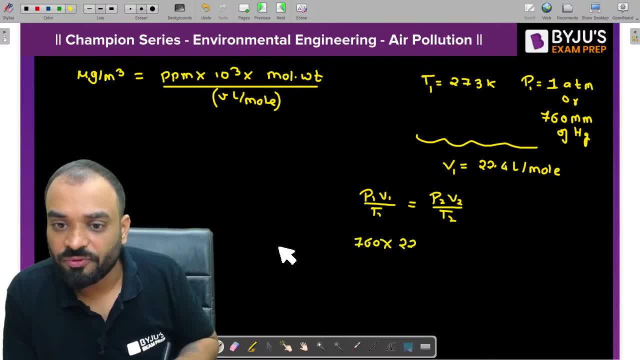 to 760 mm of Hg. V1 is equal to 22.4 divide by T1. T1 is 273 Kelvin and it should be equal to P2- P2. now tell me guys, in this particular problem they have not changed the temperature. so we will consider the same temperature, which is 760. volume is unknown to us, but the temperature. 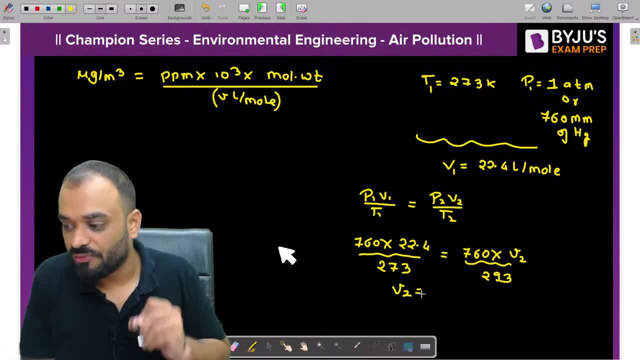 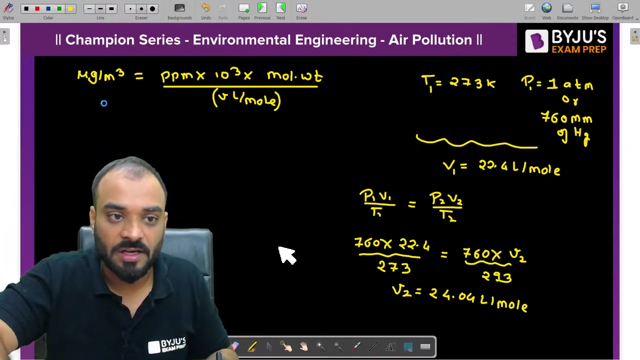 is 293 Kelvin. so please tell me, guys, what is the value of V2.. First, tell me what is the value of V2. so we are getting a value of 24.04 liter per mole as a V2 value, right? this is basically our V2 value. okay, now, guys, the concentration in. 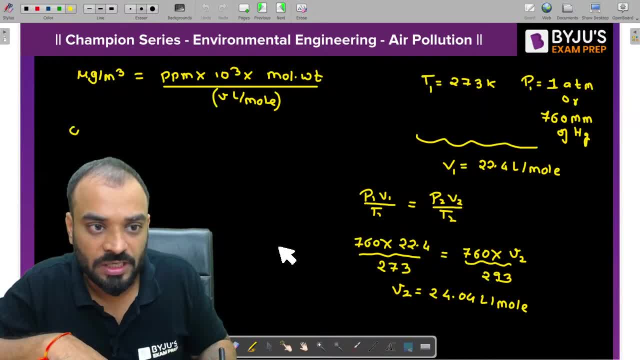 microgram per meter cube is already written, which is 0.4, so let us write here 0.4. it is equal to how much PPM? PPM Part per million? we do not know this particular value right now. let us write it as it is: 10. 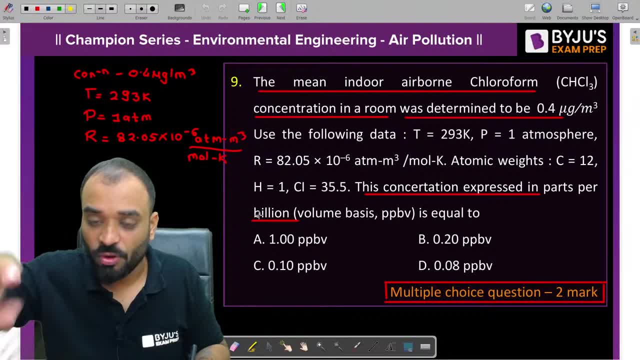 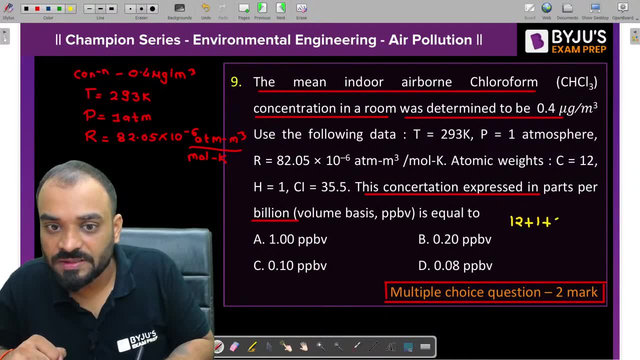 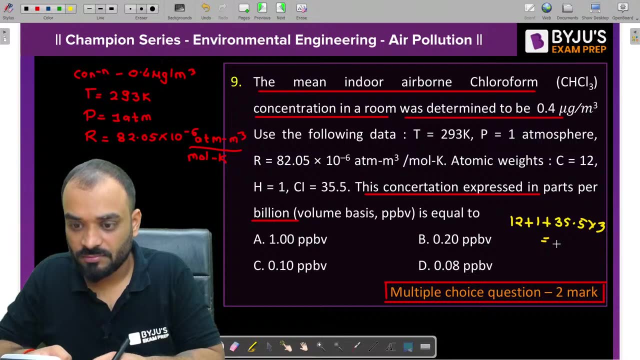 rest power: 3 multiply by molecular weight. now, what is the molecular weight of chloroform? let us calculate it. carbon is 12, hydrogen is 1 and chlorine is 35.5. multiply by 3. let us calculate how much it is. so we are getting a value of 119, I think. please calculate it. 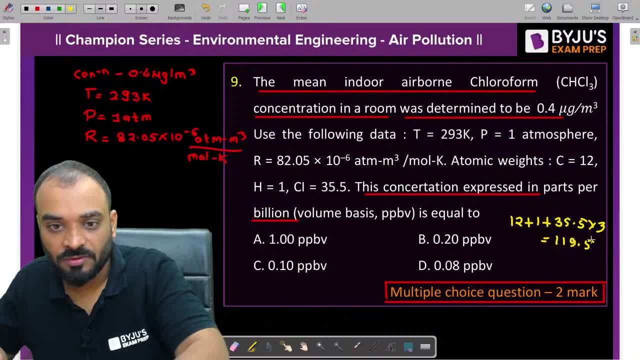 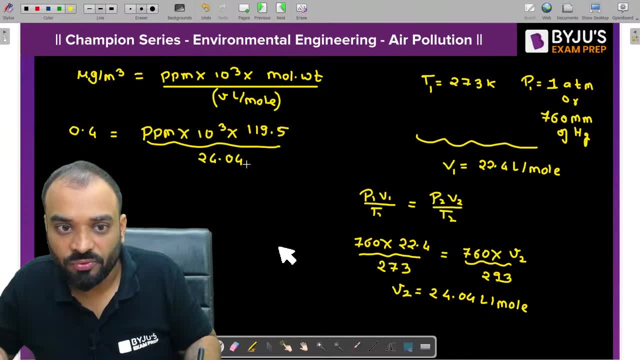 119.5.. Okay, So let us put it 119.5 divided by 24.04. please calculate the concentration in terms of part per million first. It is coming around 8.046 multiplied by 10 rest power minus 5.. 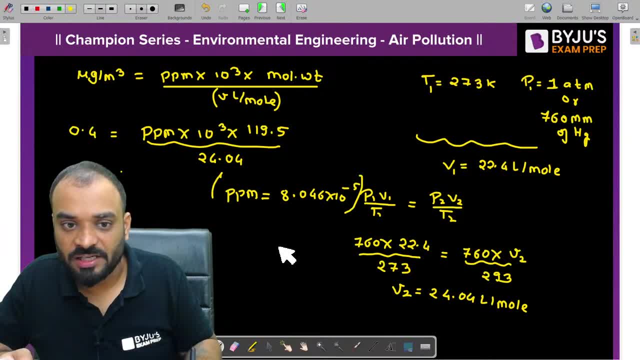 Okay, This is the value which we are getting right now in terms of part per million. now tell me, guys, I want to convert this value in terms of part per billion, so how I can convert it by dividing it by 10 rest power minus 3, right part per billion. so can I write here, guys? 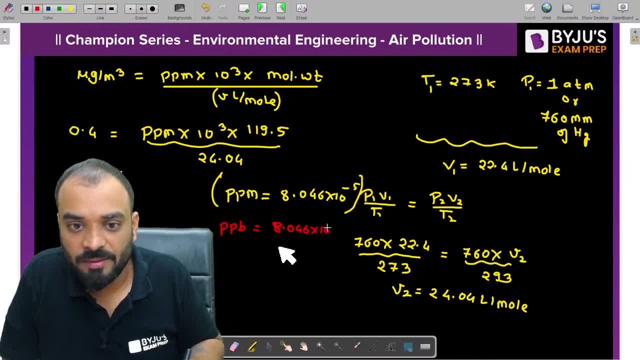 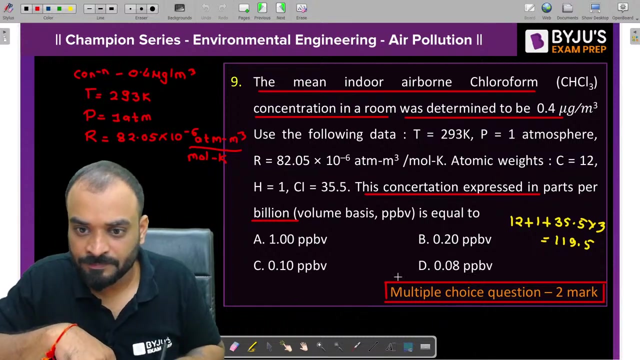 it is 8.046 multiplied by 10 rest power minus 5, divided by 10 rest power minus 3. okay, let us do it. How much we are getting? Okay, So it is coming around 0.0804 part per billion, right? so this should be the answer. d is the. 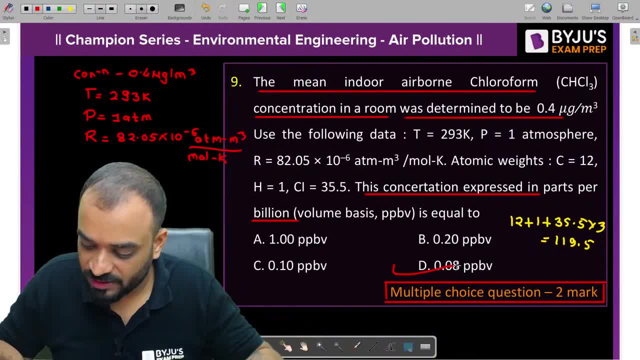 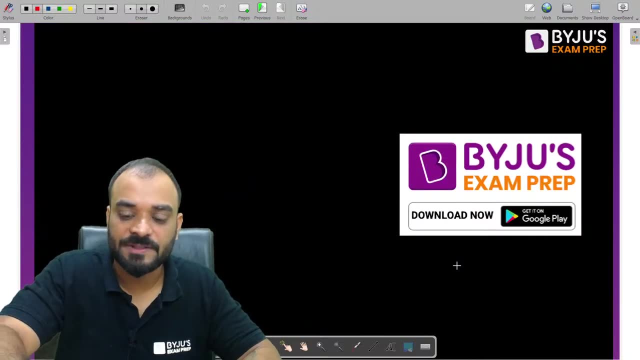 correct answer for the problem yes or no? d is the correct answer for the problem. d is the correct answer: okay, okay, so that is it, guys. that is it. so these are the question which we, I want to discuss with you for the air pollution part. but, guys, tomorrow, from tomorrow, 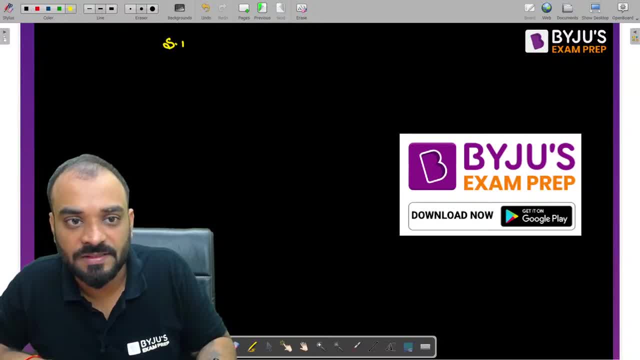 we are starting a new subject which is basically structure analysis, right, and tomorrow topic is indeterminacy, stability, right, and kinematic and static in Macy, like these type of topic are there. so we will have a session, guys, which is based upon the structure analysis. again, this subject is important, so we have three session for this particular subject also, guys. 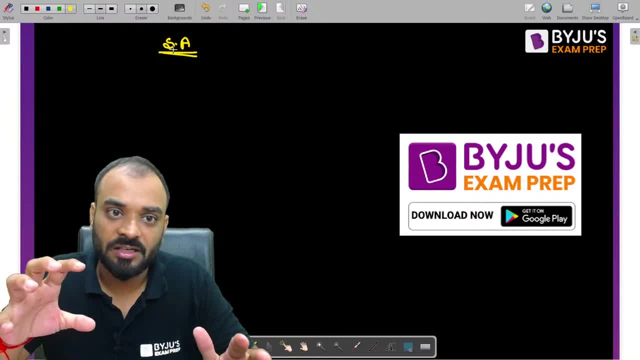 in which I will discuss: Okay, So this is a very important question and which is related to this particular subject and these question you may get in your examination also, or like, the data may be different, but the conceptual part will be same, right? so please ready for that, guys, at the same time. 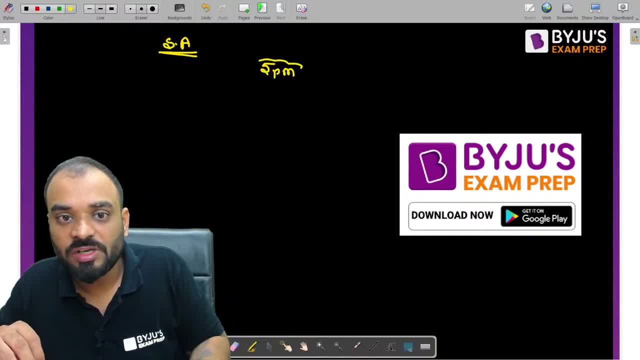 we will meet again, which is basically at 5pm. okay, you will get this particular PDF, guys, on my telegram channel, so I am sharing a link over here in the live chat box where you will get this particular link, guys and you can download this particular PDF and the previous. 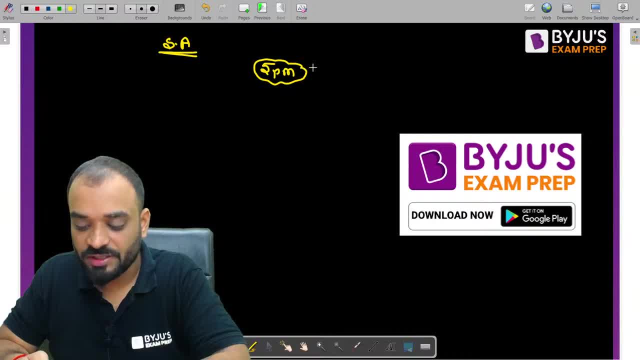 PDF also Right, Kindly join this particular telegram, guys. So any doubt, if you have, please let me know guys. any doubt, if you have, please let me know. any doubt if you have, please let me know guys. Okay, So let's meet at the same timing. but tomorrow, guys, we will start a new subject which is